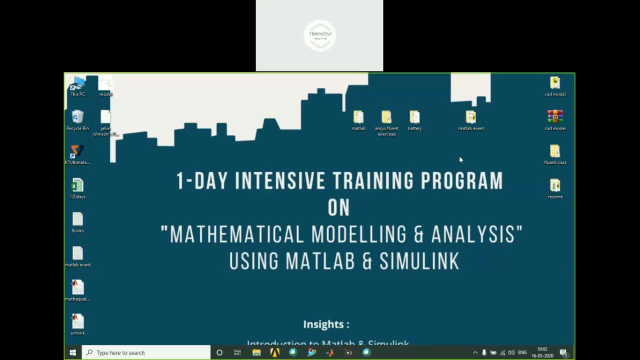 So these things are. So these things will be very efficient for you, whether you are from academy, whether you are a student, whether you are from industry, whoever you are. Okay, So, whatever things which we are going to see in today's session is going to be worth and helpful for you in your future. 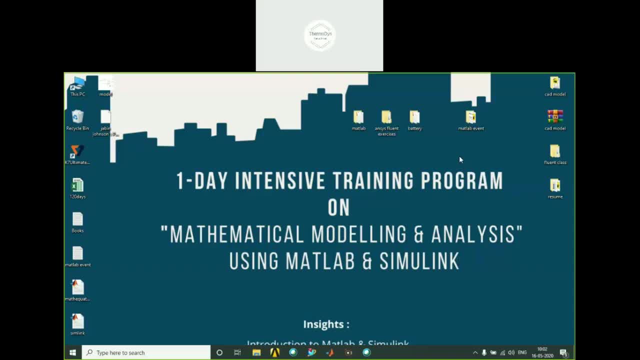 So please take a note and please write it down. If you have any queries, you are free to ask at any time. Okay, So, as I told, after 10-15. Our meeting will get locked Because you know students will come, go, come go, come go. 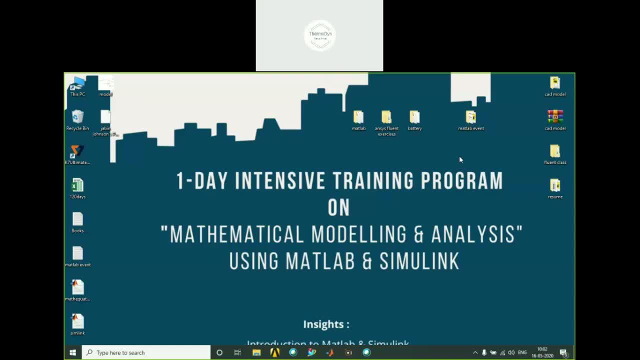 That will be a very big problem and headache for us. So automatically, after 10-15, our meeting will get locked. So after that we will not have any issue. Okay, guys, So let us start the session. 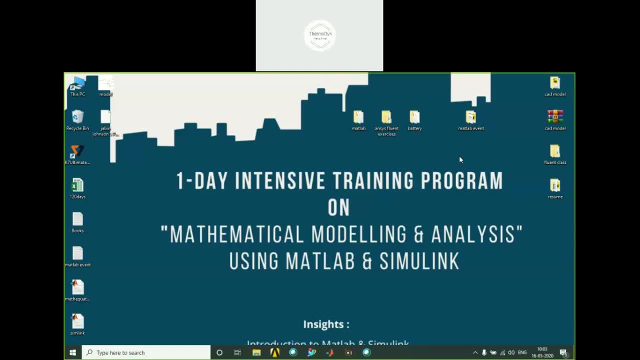 Before starting the session, I just want to introduce myself myself, Jibin, technical head Thermodyne As well. I have completed my BA, MTech and PhD in terms of thermal management. Okay, 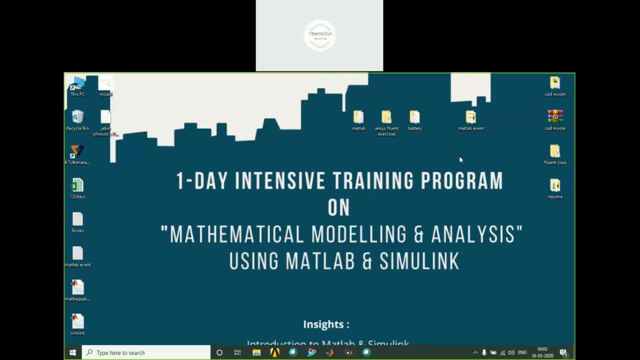 So I have also completed my MS, you know, in CFD. It's like programming kind of stuff, And a few years back I was working in a college And now I am working for NetGen solution as a CFD engineer. 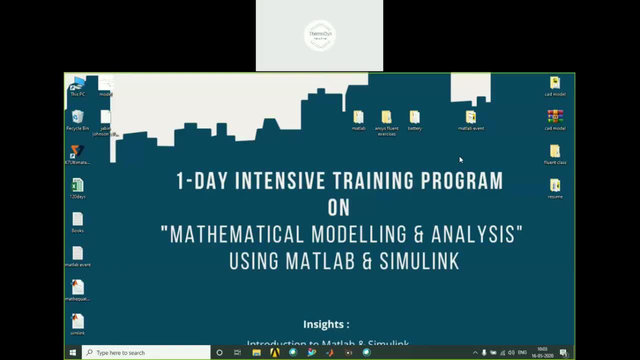 And we work on so many softwares, so many programming languages, everything. But as a motivation. I just want to tell you something. Okay, A few years back, before joining the company and all, I went to VIT University, Willur. 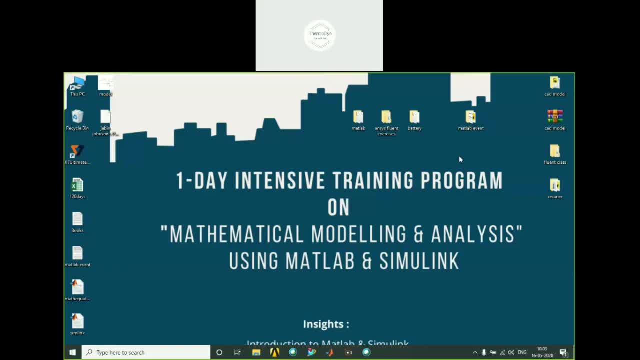 You know for an interview. That's the interview for SRF. in terms of CFD core development, Everything was fine. CFD basics, everything was fine. But finally the interviewer, the senior professor, asked me like: in which programming language are you proficient? 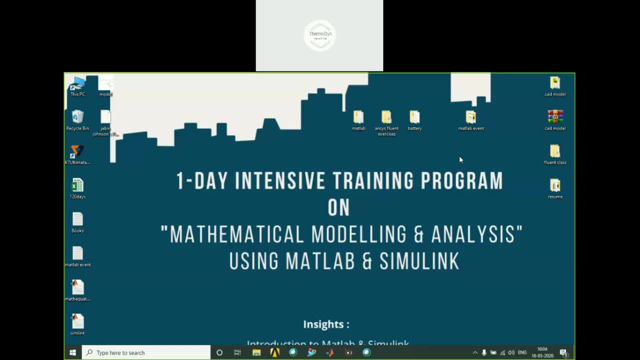 I told him I don't know any programming language. As a biology student I don't know any programming language. That's what I told him. Only because Of that reason I was not selected in that particular SRF interview. After that I realized the importance of that. 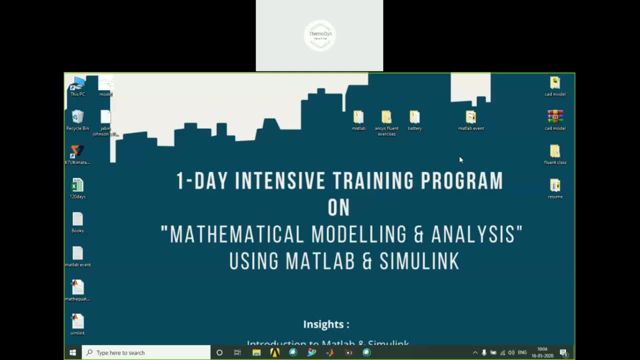 And I started to work hard on working on so many languages. Okay, So programming language In this the participants of slot 1 or slot 2, many of you asked me like how to open a MATLAB in Word. You know, it may seem funny. 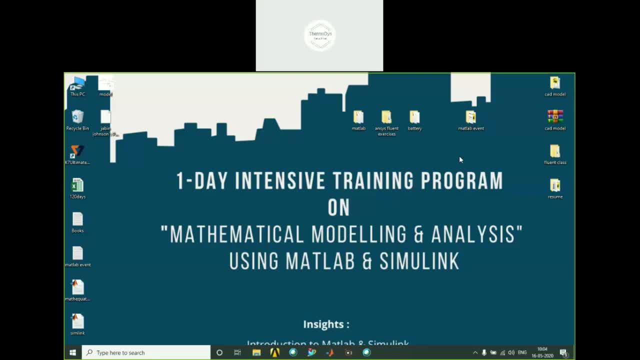 But this is the exact scenario of you know of some people. So what I'm going to do is I'm going to teach you some basic programming language skills, because programming language is a very crucial part in a career, in an academy, in a personal life. 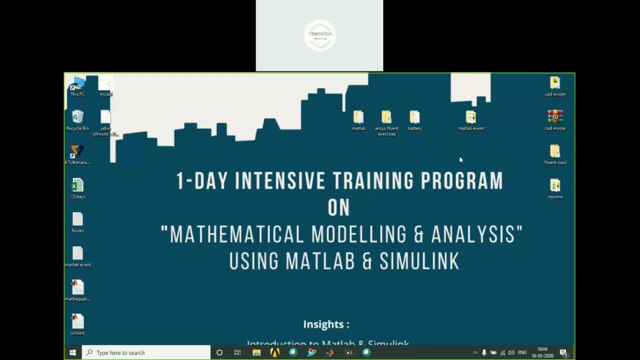 Okay. So without knowing at least some basics of some programming language, it's very difficult for us to survive in the industry as well as academy, wherever you are. Okay, So, whatever I'm going to teach you, that's going to be from basic. 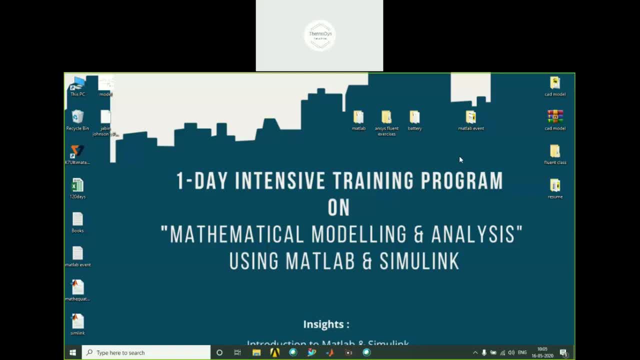 So Okay, It seems like I'm speaking so fast. Okay, No issue. I'll make it slow, because the time available for us is less, So that's why I'm just reducing unnecessary steps. Okay, So no issue. 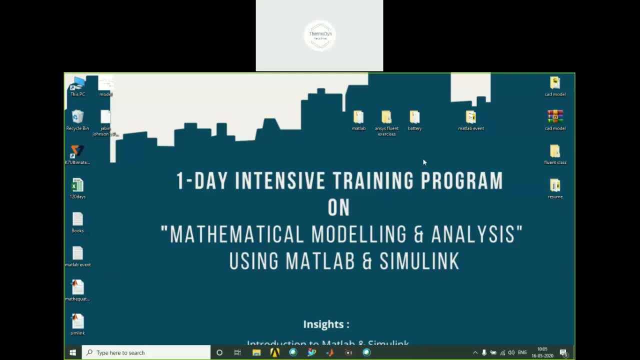 I'll take care of this. Okay, So this is the importance of programming language in whatever stream you are, Whether you are from ECE, AAA, Mechanical, or whether you are from industry, or whether you are from academy or you are a student. 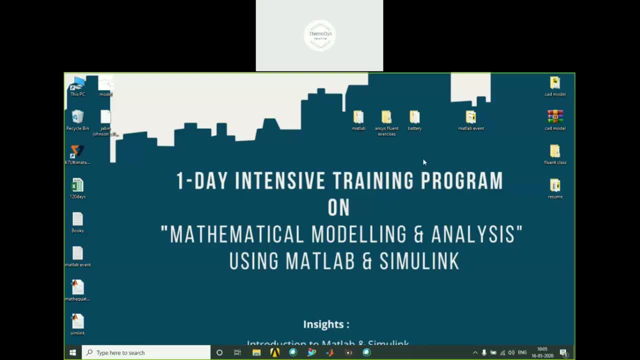 Okay, So learning a programming language, at least at a basic level, is mandatory. Okay, guys. So as of now, we have 53 participants. In second slot, we have a total of 75 participants, So let them join. 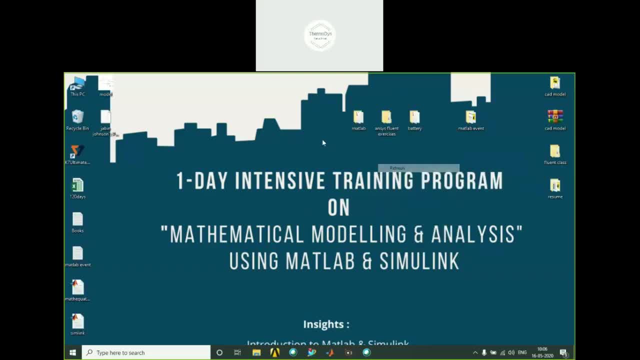 We can proceed, Okay. So first I just want to give a brief introduction on how to install a MATLAB. Okay, So we have SHAD. We have two links: One is of MATLAB 2019, and another one is of MATLAB 2014b. 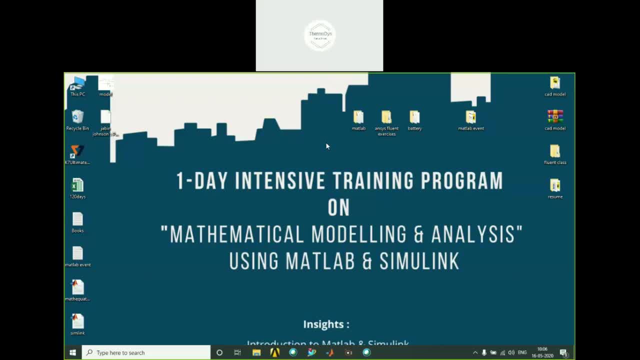 So there is a particular reason for me to share two links. Okay, If you have a very good system with a very good configuration, please go on with MATLAB 2019 version. MATLAB 2019 version: Okay, Okay, Because 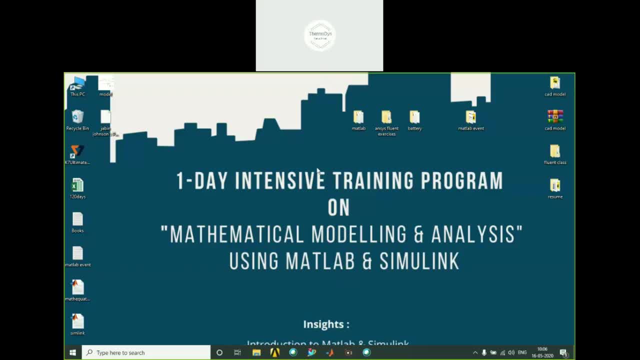 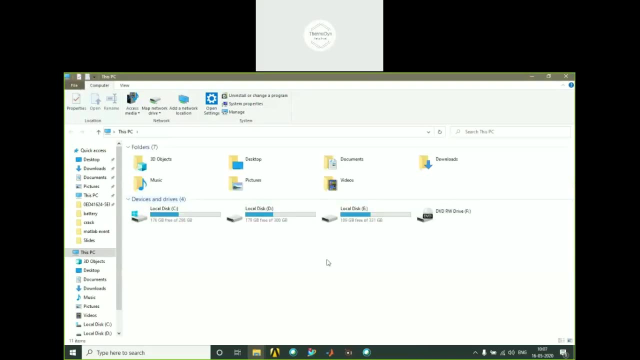 It has so many advanced features for simulink modeling. Mr Dhinadayalan, you are asking me annotation request, So please don't send me those requests. Yes, And I have SHADU MATLAB 2014b. That is because that is a very standard version of the MATLAB. 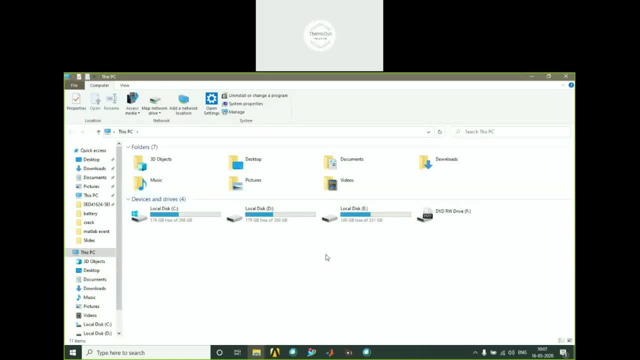 Okay, That is a very standard, very simple, very lightweight version of the MATLAB 2014b. Okay, So I will show you how to install MATLAB 2014 now. It is very simple, Okay, So please see. 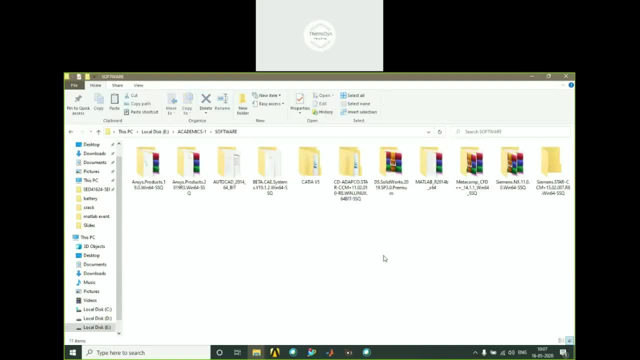 Just go for your software directory. Just go for MATLAB 2014.. Okay, So after downloading, you will only have WinRAR file. Okay, That is a compressed file format, So just extract it. You will get something like this: 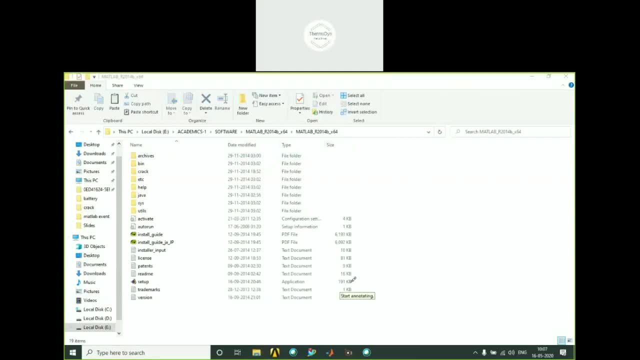 Guys, please take a look here. setup, So just click on the setup, right click, just run as administrator. Okay, very simple in terms of installation. So just run as administrator. After clicking run as administrator, it will ask you some. next, next and all. Okay, just give next and it will ask you some. it will ask you to install license key. 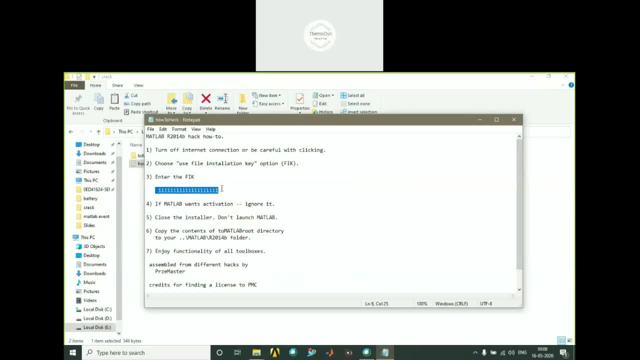 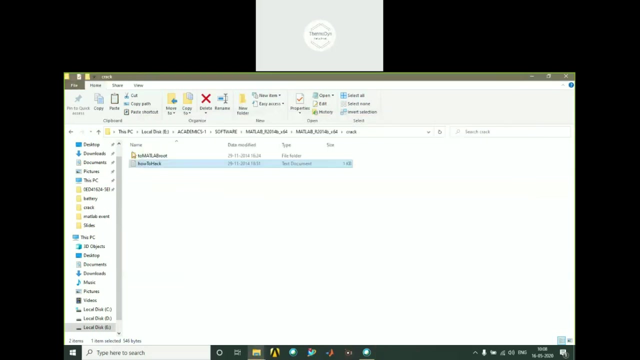 In that place please enter all one. Okay, some of you have asked me give us a license keys like that. So in that place please use all these ones and give next and give finish. So the MATLAB installation. it will show you like the MATLAB installation is successful. After getting a successful screen, please copy the contents from this folder. It is, like you know, to MATLAB root. 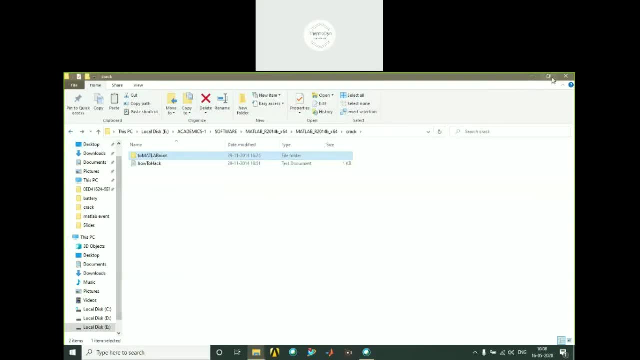 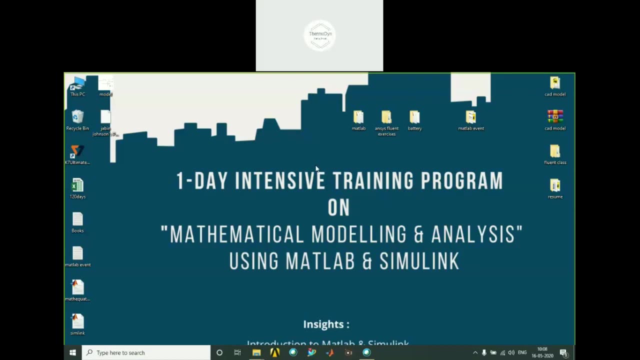 And Put it in your C folder. That's all. So just run the setup, Just put a installation key- It's, like you know, simple, one, one one, and just give next. next, Once you get a successful screen, just copy the content from the crack folder to your C direct. Okay, so this is simple way of installation And after this event we will share you academic version. Okay, so academic version of the MATLAB installation. 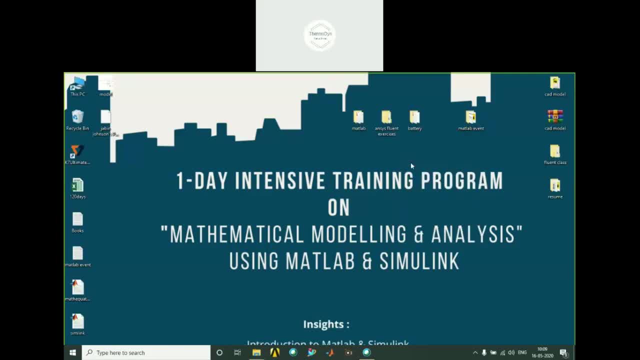 matlab so that you can download it. you can install it with your college id, with your whatever it is, whatever you have. okay, so that is available for you for the period of one year, or else you can use, uh, the links which we have provided. okay, so the okay, so that's all. 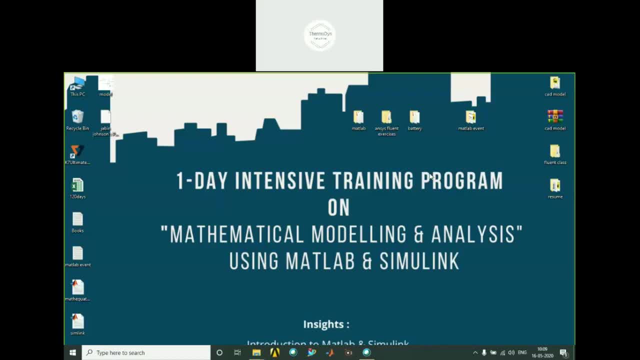 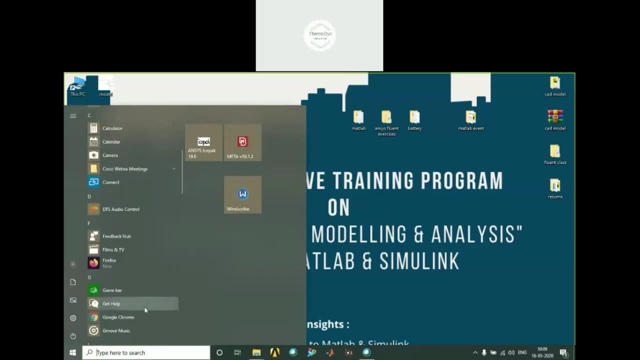 all you know regarding uh installation at all. so we will start a session now. uh, guys, once you have installed your matlab, what you have to do is just you can go for all programs, in that you will be able to find your matlab stuff. uh, since we have already installed. 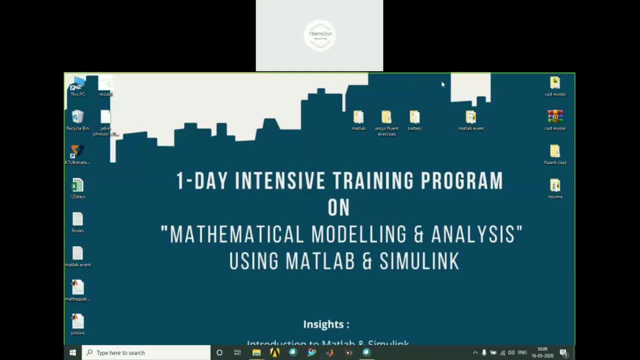 katy gain, you are getting 2019. that we will see that, uh, later. okay, so since we have installed that earlier, we i have a link over here, matlab link over here. okay, so just click on that link. okay, so it will get opened. so why we have chosen MATLAB? 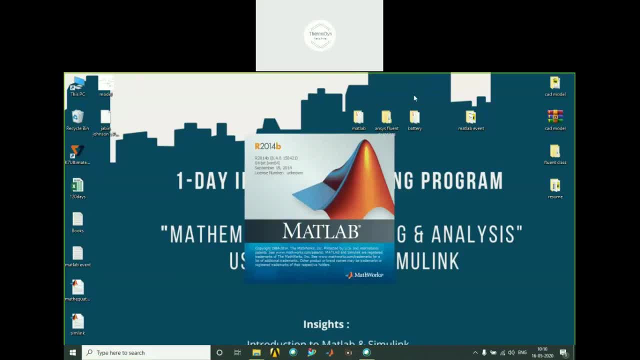 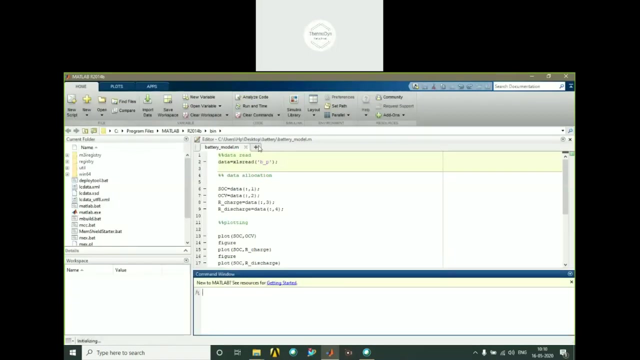 now in industry we have two major programming language. one is MATLAB, another one is Python. but as far as academy people are concerned, like from ECE, EEE, mechanical MATLAB is a very high level as well. very useful programming language than Python. okay, so if I say than Python, Python is very useful for. 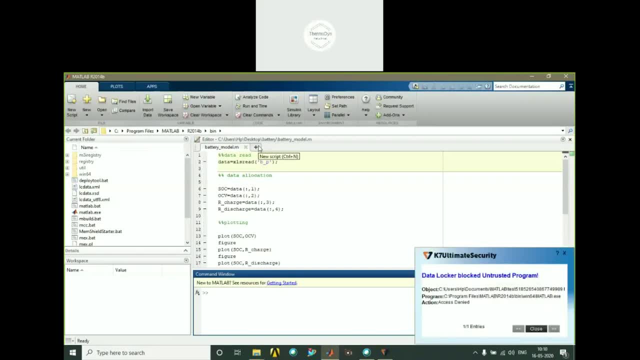 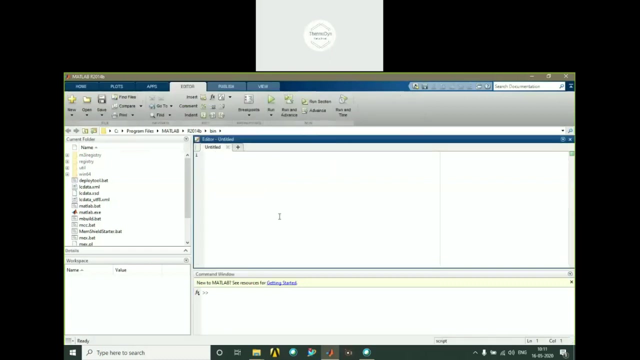 computer science or, like you know, data science, like that, but in terms of mechanical or ECE, as far as academy people are concerned, using Python is bit. you know, that's not that much relevant, so that's why we have chosen MATLAB. okay, guys, so this is our battery model, but we are going to see you can just close it, okay. 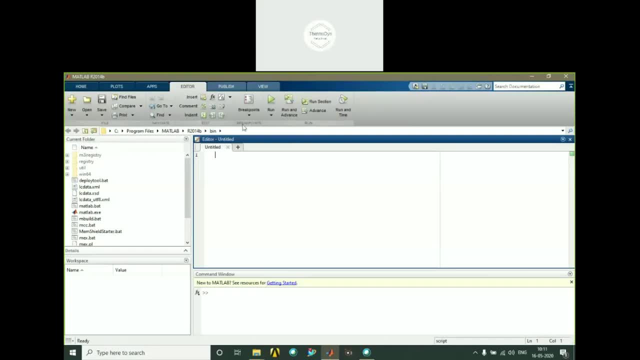 so this is how, once you open a MATLAB, you will get a user interface kind of stuff. okay, so some of you may feel like completely new to this interface and some of you may feel, see, like you have already know the stuff, but somehow we will be able to use MATLAB. and some of you may feel like completely new to this interface and some of you may feel, see, like you have already know the stuff, but somehow we will. 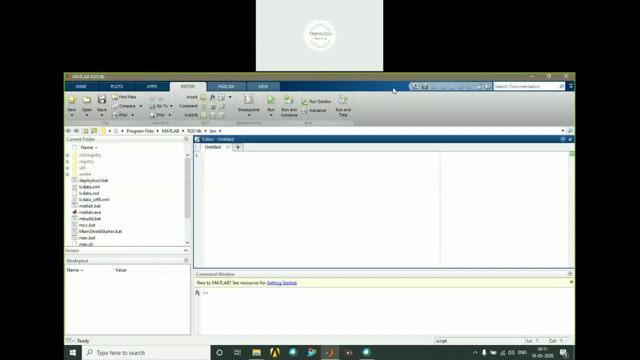 teach you from the basic. so, guys, please listen, as I already told, please take a note and please write down all the things which we saw, which we see, okay, so first I'll take some few minutes to explain the interface of the MATLAB. so first I'll go for home. okay, in the home you will have so many stuffs in the 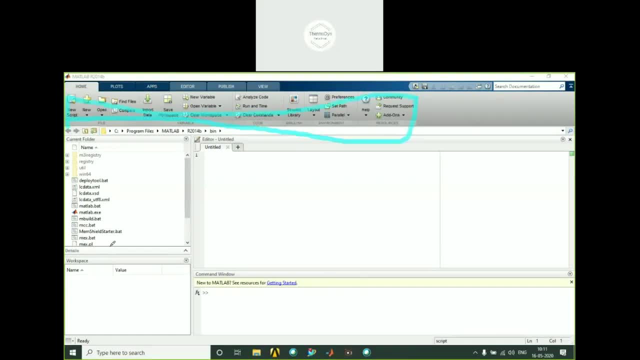 interface. I'll take some red color. okay, so you will have so many stuffs above, below right side, everywhere. but what is the use of all those? so all the stuffs here, except Simulink library, you know, can be accessed. we are just code, simple code, okay, so there is no need for. 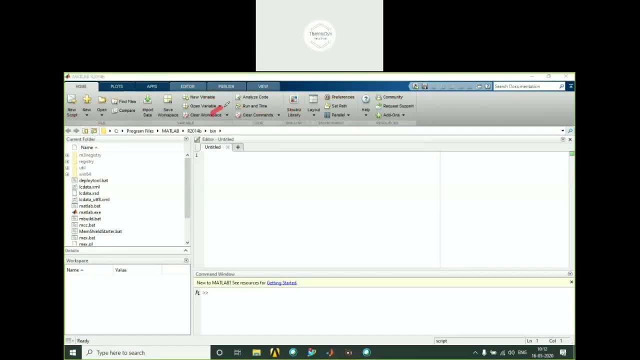 us to go here each time. use all these options to run, check, assimilate our program. okay, for doing all these tabs, we have a simple matlab codes. so always, we will add that to matlab code. are not uh icons like here? okay, so, most of the time, in order to work on simulink, i'll be using a simulink library. okay so, but in order to write, 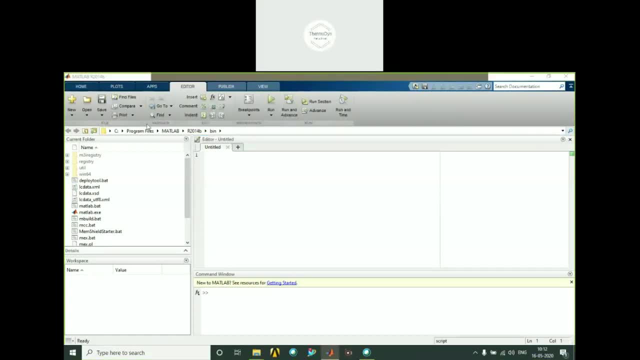 a script in matlab. uh, i'll be. uh, you know i'll be using most of the time editor window, okay, guys. so in the left side you will have something called current folder. so current folder is nothing but the folder in which you are saving your uh matlab script, m script. okay, 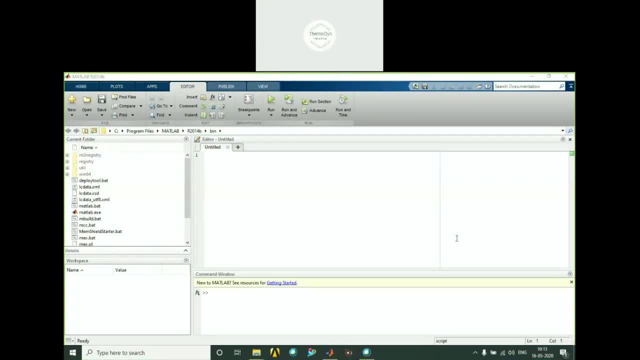 so, guys, you are facing audio trouble, but none of us have complained regarding that. so you have a command window, you have a workspace, so you have workspace. so in workspace, all your data, like if you define a equal to 1, a equal to 3, so whatever it is, whatever value you define, whatever 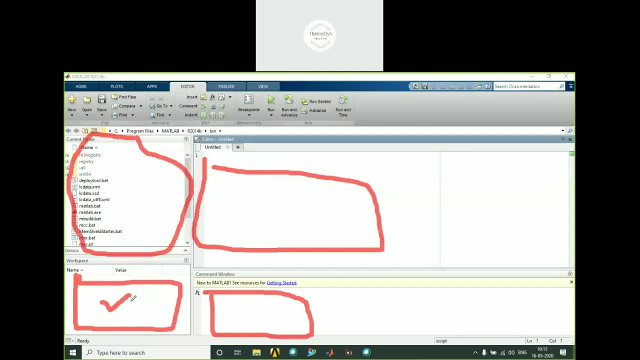 matrix you define. it will be a current folder. so you have a command window, you have a workspace. it will be, you know, stored in this particular place. okay so, and whatever command you are going to run, like clear, clc, close, all, whatever, so excel, street, whatever you are, if you are going to read, 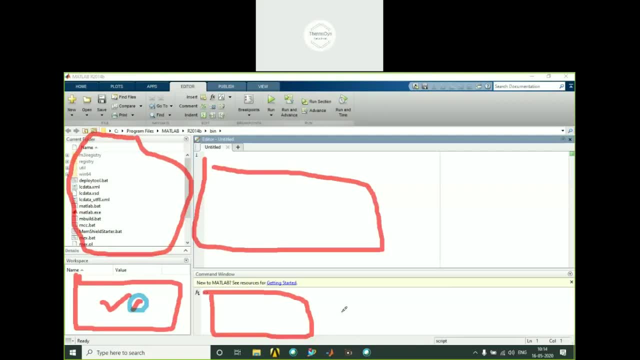 uh, excel data. you are going to use excel x, excel street. whatever command you are going to run, you are going to put that command over here in this particular space, okay, so, if you are going to write a script, then you are going to use this editor window, okay so. 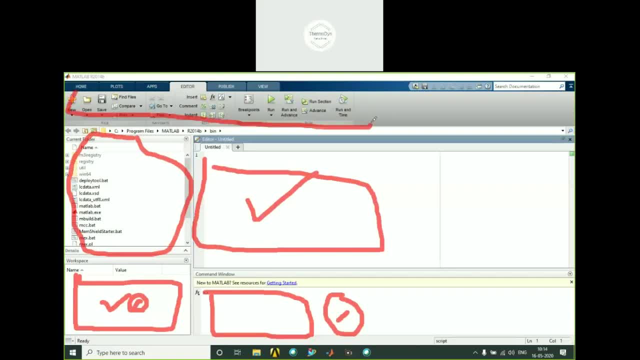 yes, please look at the screen. all these stuffs can be accessed via codes. if you want to write a script file, you are going to use editor window. if you are going to run some command, you are going to use command window. if you are going to define a variable, you. 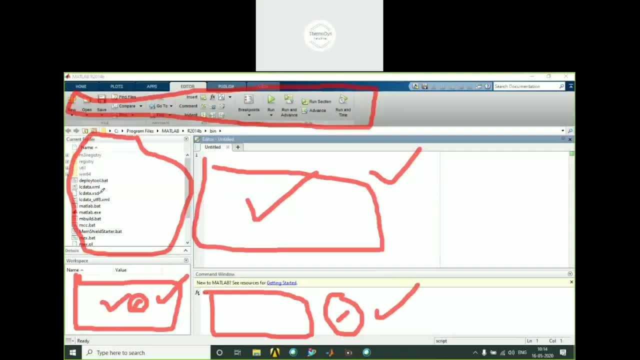 are going to use this place and- and guys, please make a note- most of the time in matlab we used to address some external files, some function file, some script or some other stuff. you also want to add some Third- coses. on shuttle lab, they actually imagined a variable to use and we are going to Фbaby. most of the time in matlab, we use to address some external files, some functions. we are also wee to add some drauf. we are going to do command and aingua, and let me, so, let me, défiENc. oh bye guys, please keep the. You'll see what you can understand this. I M cesRA knew that you. preventing test. 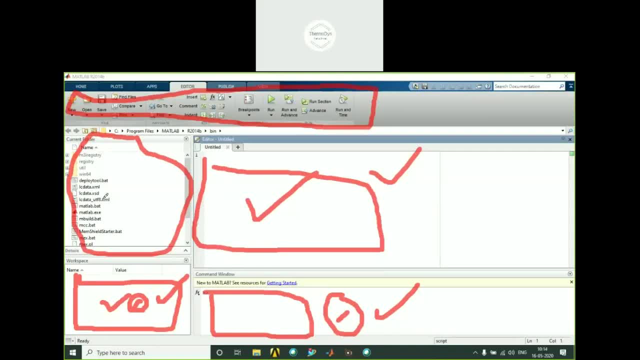 file, some script file, some excel file, some data file, whatever it is. so matlab cannot just search your whole laptop or system and can find the file, okay. so whatever file you want the matlab to access, please put those file in your current folder so that it can easily access it, okay. 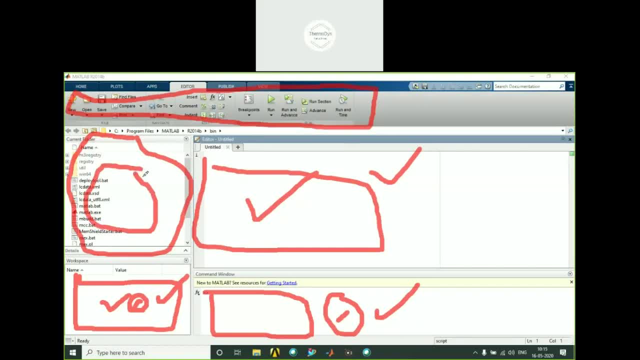 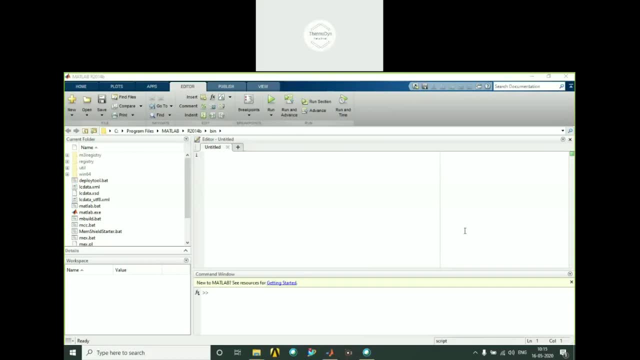 and the time required to run the program will be short. okay, guys, so this is all about, uh, you know, a matlab user interface. i hope you understood, but you know this is not all. this is just a one percent of our program content. okay, so fine. so i'll move on to some programming syntax. 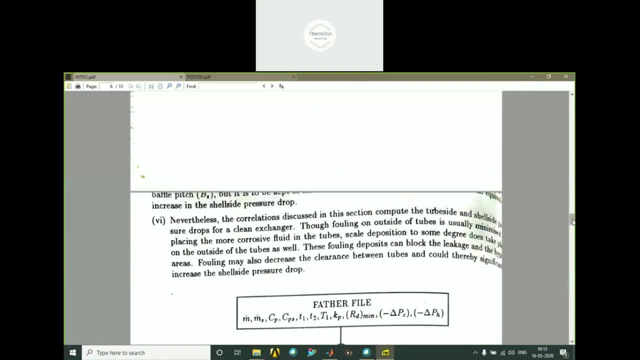 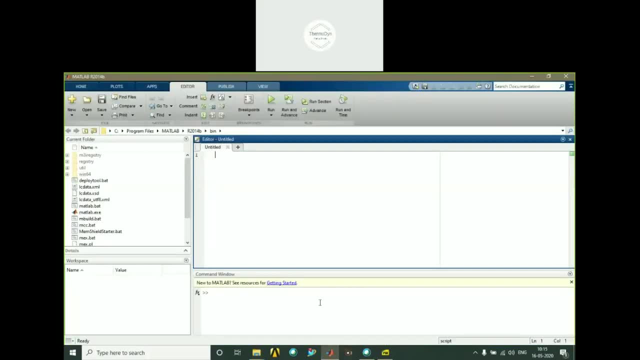 so we have uh scanned some matlab nodes. okay, so before uh moving on to intensive coding or simulink model generation, uh, i just want you to know: how does the matlab code look like? okay, so how does the professional matlab code look like? what are the contents in it? 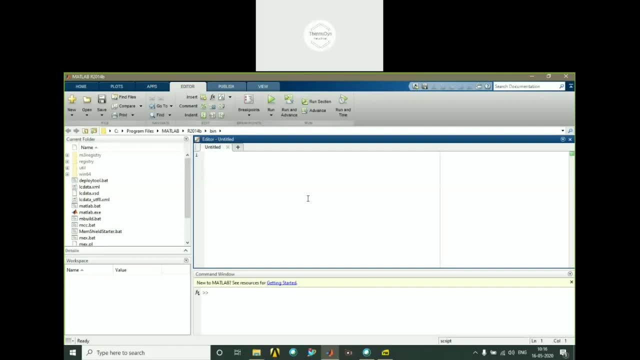 yes, so, uh, what are the contents in it? what are the meanings for all? how to clear the screen? everything you should know, because most of you are from college or from academic without any prior knowledge, guys. okay, so i'll be telling everything in basic, so please be patient, but these things will be of. 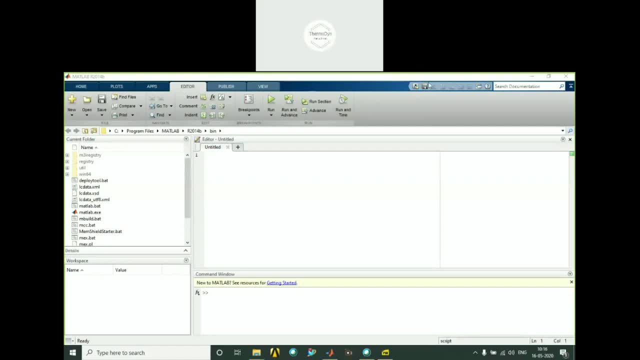 very important for you. okay, so, yes, so, most of the participants have no issue with the audio. you can have any issue please in the meeting. go out, come in, it will be fine. okay so, okay, guys. so first i just want to make sure, uh, please see here, still now, i have not, uh, provided a proper. 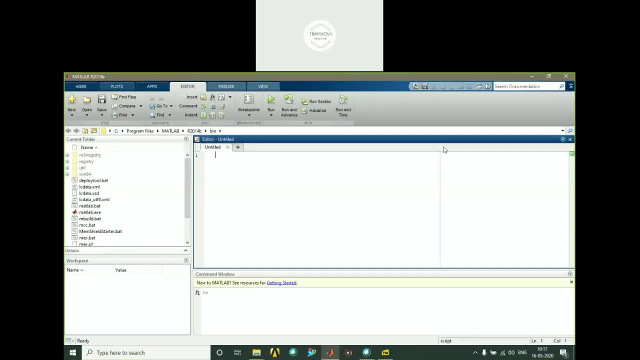 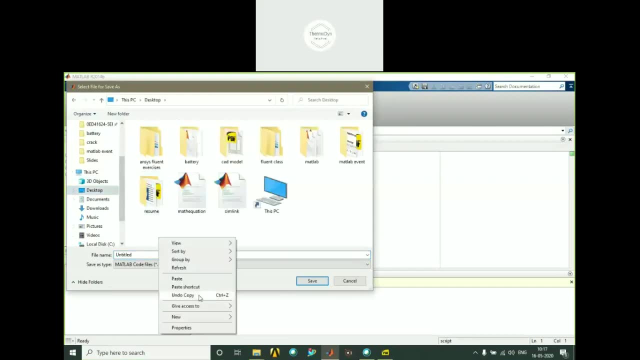 title for my code. okay. so, in order to provide a proper code, just go for save us in the desktop. i'm going to create a new folder that is going to be my current folder, program one. so, guys, uh, please make a note in matlab, whether it is in title or, uh, wherever it is. 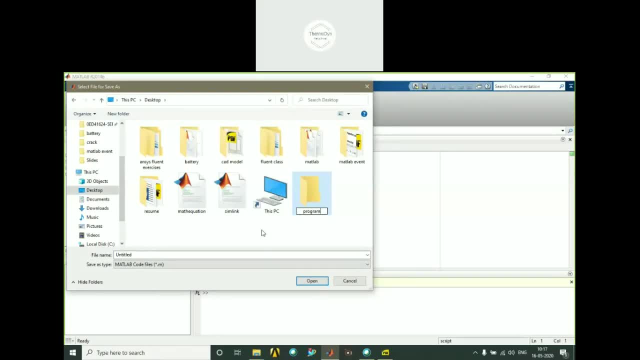 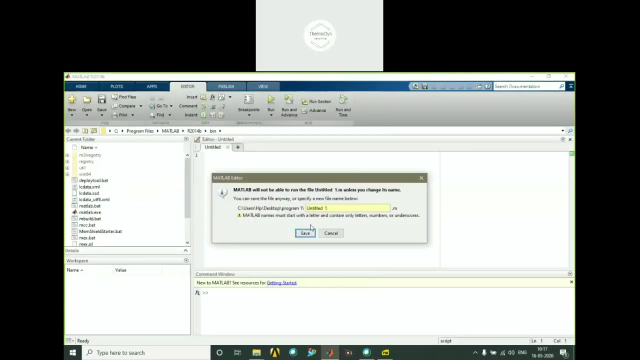 you are not supposed to use space, okay. so space is a important uh function in matlab, so unnecessarily you are not supposed to use space. that is applicable even for you know uh title. okay, so i'll just put program one. i'll go into program one. if i give unnecessary space, what happens? so if i save it, it will show me some error, okay, so 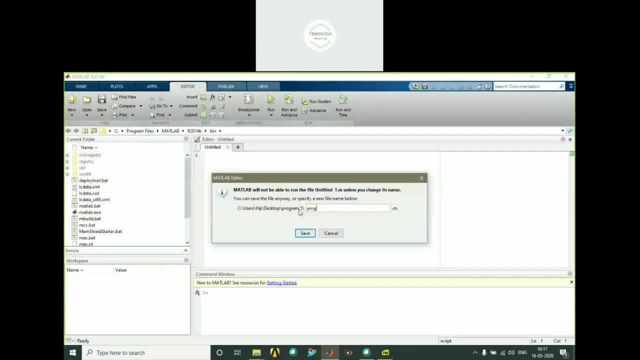 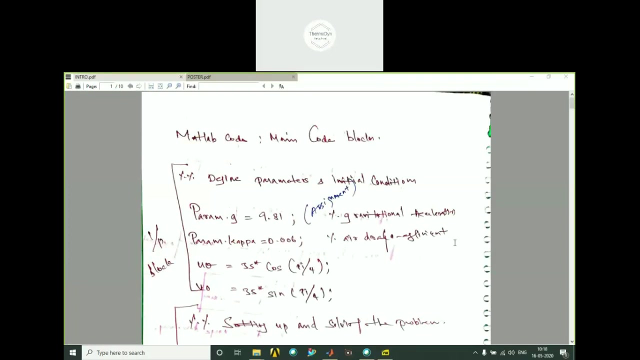 i'll just delete this. i'll put program prog underscore one. just save it. okay. so this is our very first program and very basic intro. okay, so, guys, now i'll explain you uh different blocks in matlab. okay, so matlab code basically will consist of uh major applications of matlab. so i would like to say like uh, major applications in the sense, um. 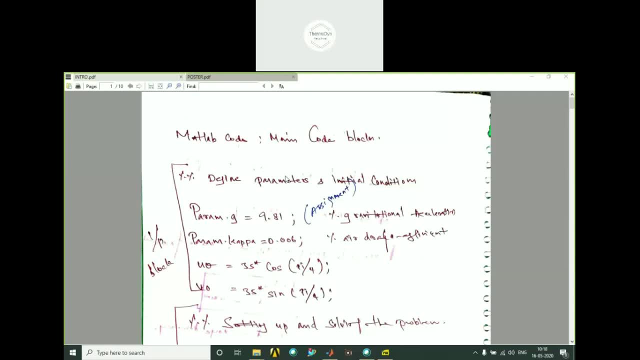 wherever it is, whether you are from computer science background, whether you are from rnd background, whether you are from triple e, mechanical, wherever, whatever your background is, uh, you know, uh, you'll be using matlab. uh, most probably you, uh, if you are not using some programming language. uh, 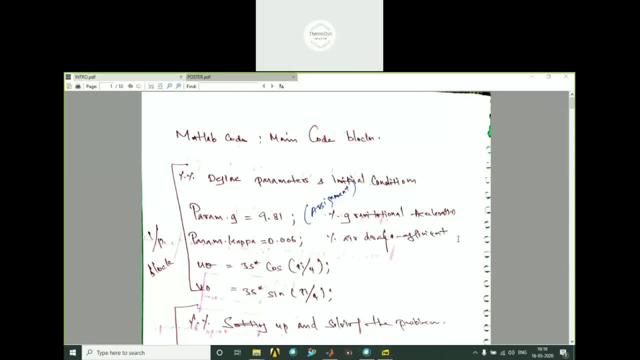 some of the students are facing guys. uh, please make sure, is my voice audible? effects? please put s. i hope you can see. yes, good, uh, most of the participants have no trouble with audio. if you have issue, please check your stuff. okay, okay, guys. so, as you asked, dina dylan: uh, wherever you are from, whether you're 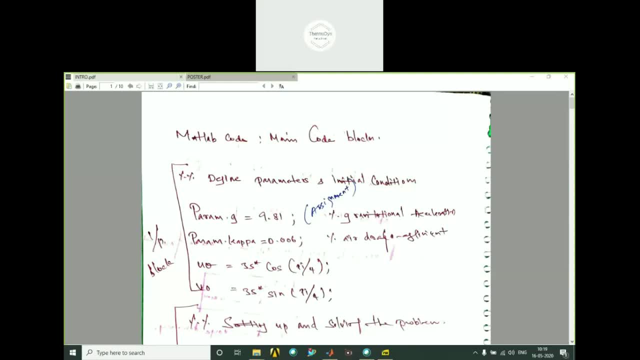 from industry, whether you are from academy, wherever uh department you are from, it doesn't matter. okay, so matlab, or any programming language, lays the very basic foundation for understanding as well, making the thing simpler. okay, so we will solve some problem so that you itself, you yourself, will find the importance of the program okay, so yeah, 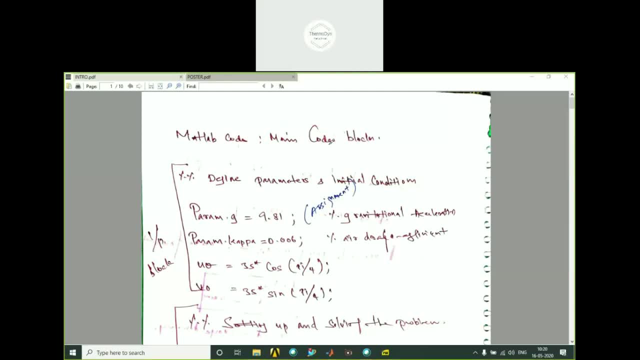 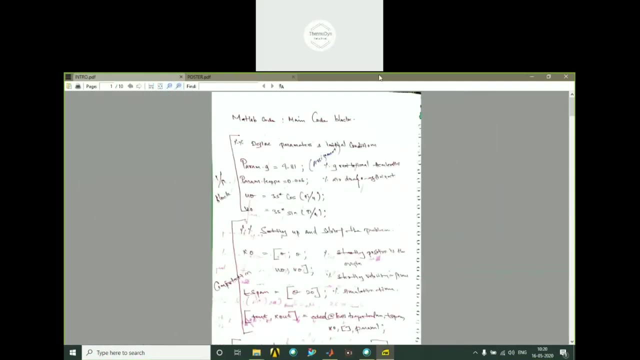 let us proceed. so this is the thing which is displayed in your screen is a very basic, you know, blocks of a MATLAB code, typical MATLAB code. actually, our code will have a three major blocks, guys. so first one is input block. okay, so input block. input block means like in C language: first you define all the 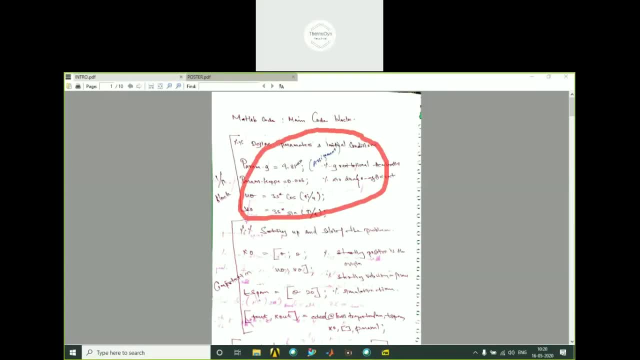 integers. okay, likewise in the MATLAB. first we have to define all the values, because any programming language will not identify your variable. if you are putting a, B, you only can know the value for it. okay, so before proceeding into your formulae formulae or your loopings, everything first make sure that you are entering all the 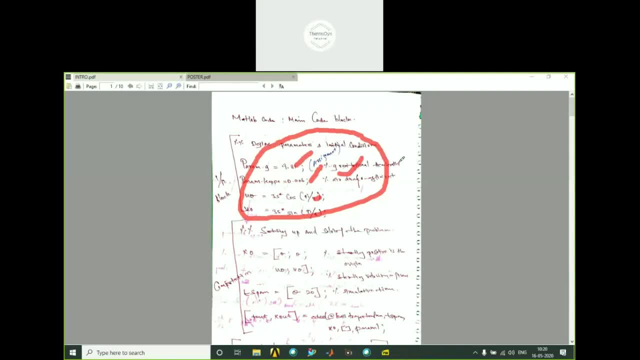 unknown variables. you are defining variables for all the constants or whatever it is you are going to use throughout your program. okay, so first block deals with how to define the variables in MATLAB. okay, that is known as input block. next one is computation block. this is where the heart of the MATLAB. 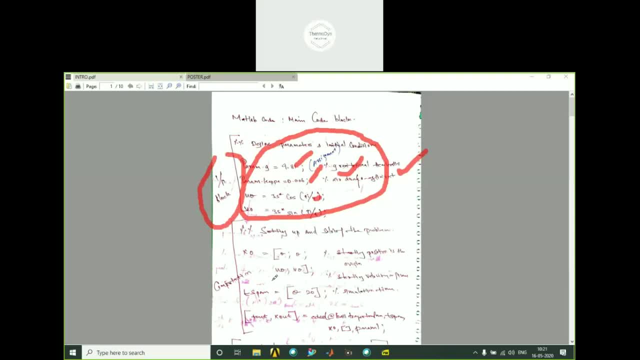 code is okay. so it's like: whatever problem you are going to solve, whether you are going to carry out a regression analysis, statistical analysis, or whether you are going to solve the heat, heat transfer problem, whether you are going to write a web application, whatever, it is okay. so the formulas which you are 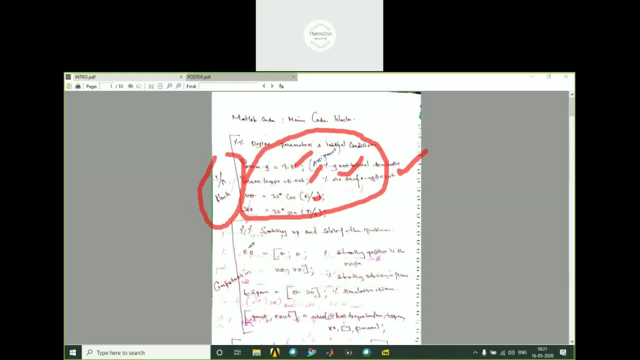 going to use for all your individual application. you are going to put it over here, okay, so I'll take one example how. I'll show you how to rearrange the formulas to put it in the MATLAB shortly, okay. so after that, once you have included a computation block, once you have included 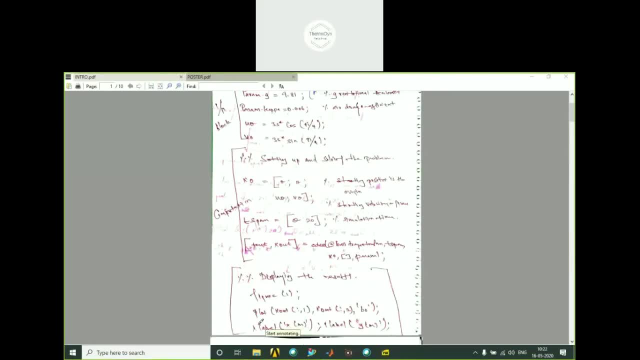 a computation block. next is like a post-processing, so we have to take out the results and show, like in form of graph, in form of, you know, image, something like that. okay, so first block is like input block, next one computation, next one output. okay, very simple syntax: input solve output, okay, you know. in addition, 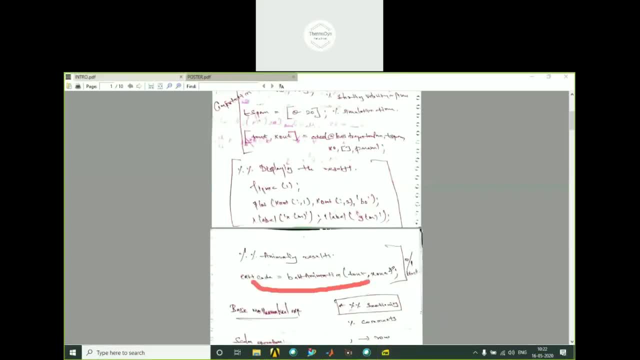 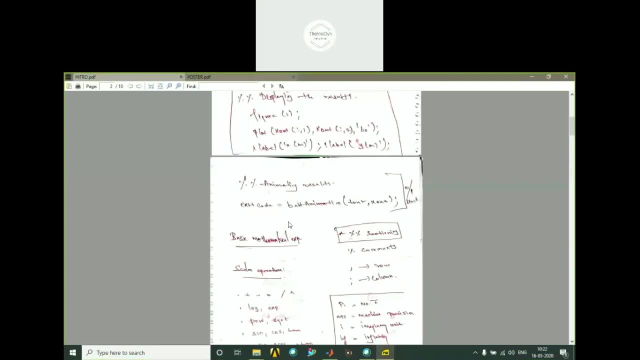 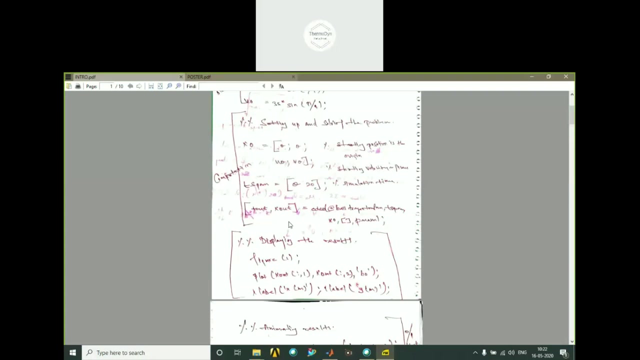 to this, you can even animate the results. okay, that is also a form of taking output. okay. so, everything we are going to see shortly. so, guys, in this particular session, in this particular day, we are going to see major stuffs. I'll explain all the things which we are going to see now. first one is importance. 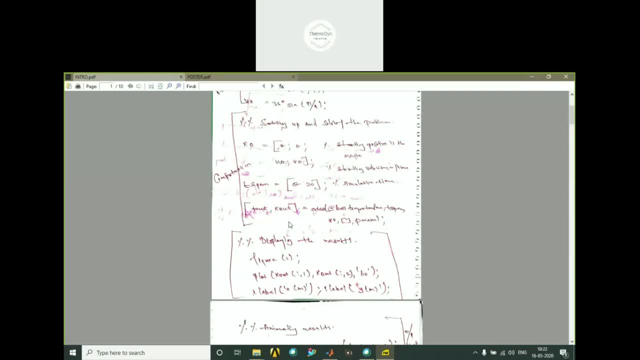 of MATLAB. okay, so it's like carrying out, that is, this operation, and how powerful the MATLAB is. the next one is: we are going to write to simple program program and we are and I'm going to show you how to solve and heat exchanger problem. okay, 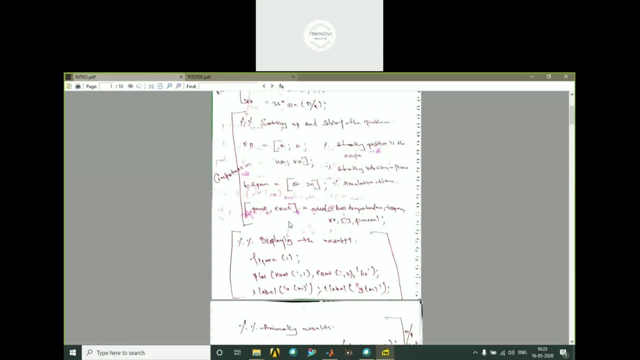 so, after seeing all those, we are moving on to simulink part. so I'm going to show you how to fix problem after sehenGSа to create- or you know how to create- a sine wave or pulse generator, a kind of stuff, simulink- how to add the signals. no, actually there is no video playing. 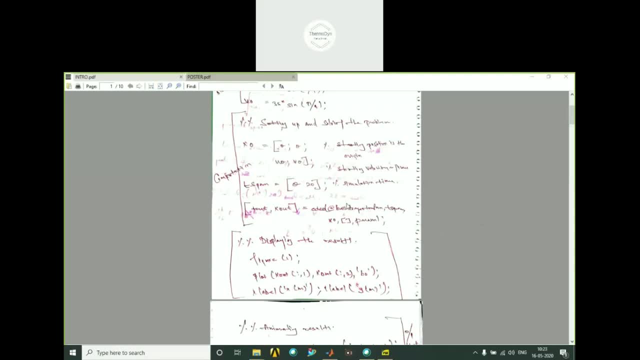 no, actually I'm showing one screen. it's not got stick, so please don't get confused and confuse others. okay, so I will show you how to generate a different pulses, sine waves, different waves in simulink, how to add it, how to display it- a lot of first of sudden, and after that I will show you how to solve. 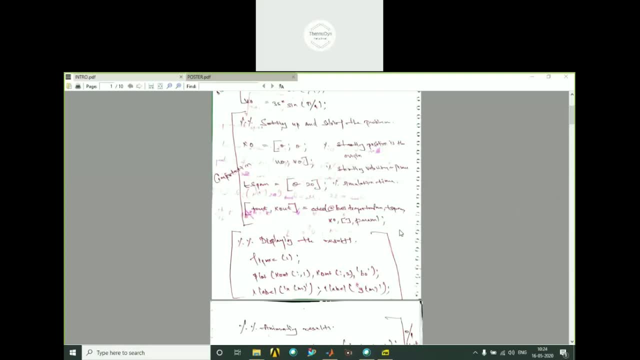 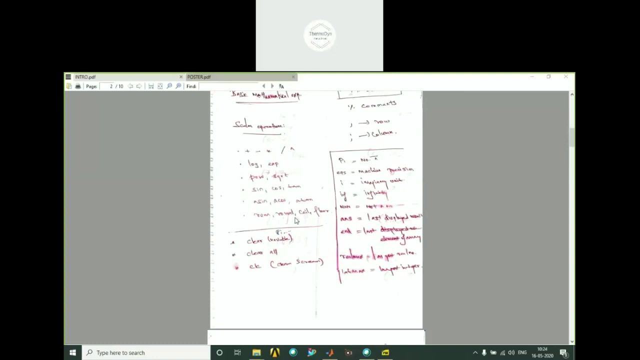 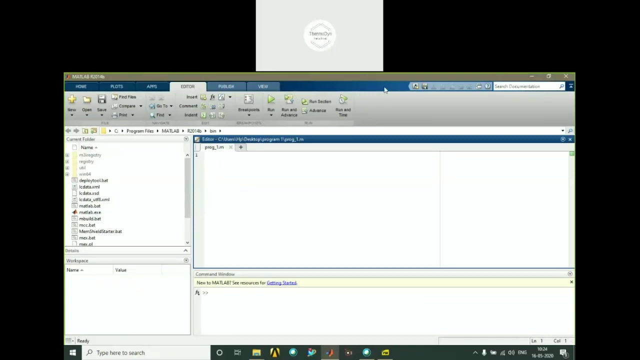 a equation, mathematical equation, using simulink. okay, and after that I will show you how to build a battery model. okay, okay. so all these stuffs we are going to see shortly, so please stay a lot s guys. so now I will move on to our program 1. okay, so, yes. so first, as you have noticed in 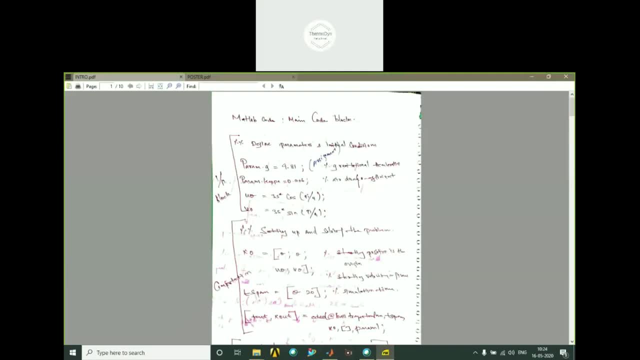 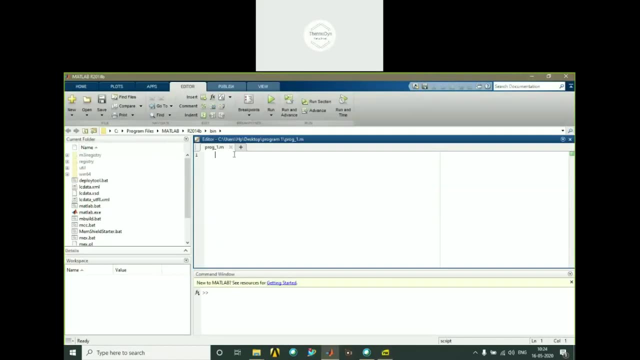 your in the PD of PDF. we have our three blocks: no input block, computation block and output block. so before starting any MATLAB code, it is necessary for us to use three lines. okay, that is clc, close, all clear, all okay. so why we have to use? what is the significance? 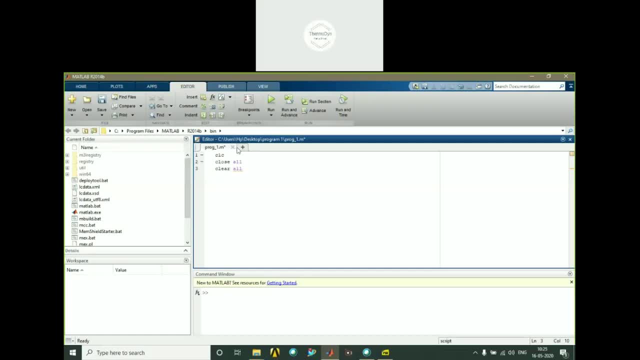 of these three commands, first one is clc guys. so whatever stuff you have in the command window, okay. whatever stuff you have in the command window in order to clear that you will be using clc, okay, because you will be running codes of, you know, even thousand two. 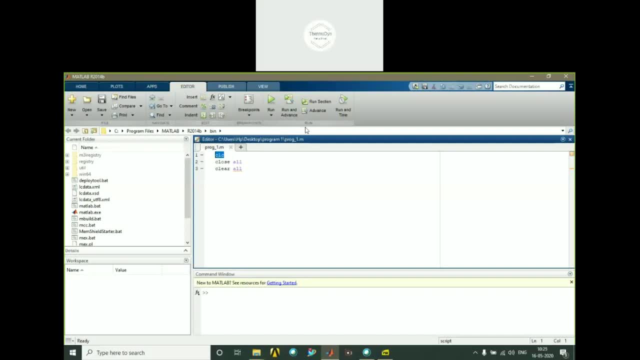 thousand lines and from each and every lines you will get output generated. so in order to clear everything from a command window, we have to use clc. next is close. all so close. all in the sense, as i shown you, you will be generating different fields in the command. 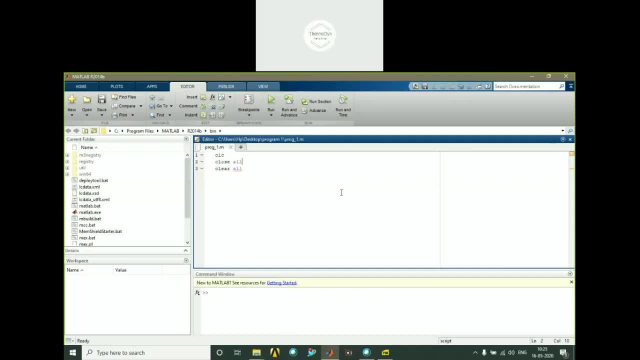 windows, different key figures, different graphs, different animation plots, tr pane, everything. okay. so instead, until or unless you close everything, it will be visible as a separate window in a MATLAB. hold on, sorry, how do you do this? okay, so, before proceeding to a new program, close all those old janbs. so, in order to close all those files you are suppose to, 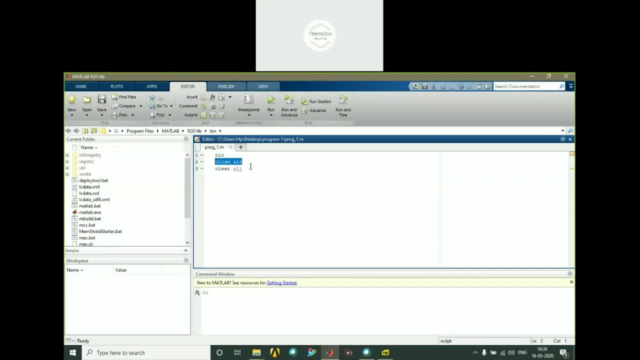 use close all. okay, so we are suppose to use close all in order to close all the external files like uh, plot files, display files or else close all. so we are suppose to use close all to close all our files secure So effectively. what we have to do here is we have to secure. 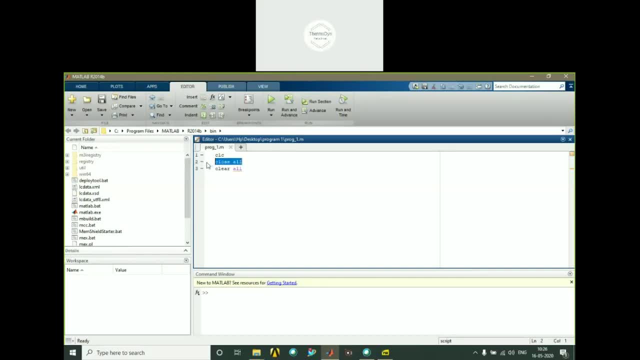 you know animation file. so in order to close all those you will be using, uh, close all uh and clear all. so uh, i will not just recite the things orally, i will even show these uh things. okay, so listen. okay. so why we use clear all? so we use clear all in order to clear the workspace, okay. 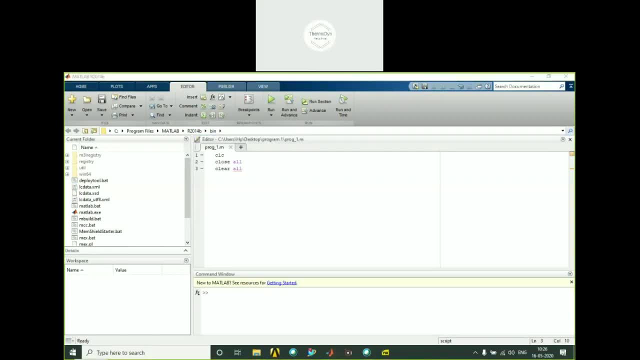 because whenever you assign a value, a equal to one, a equal to two, whatever it is, uh, it will get assigned over here. in order to clear my workspace, i'll use clear, all okay. so the first one is to clear my command window. next one is to close all my unnecessary windows external to the matlab and 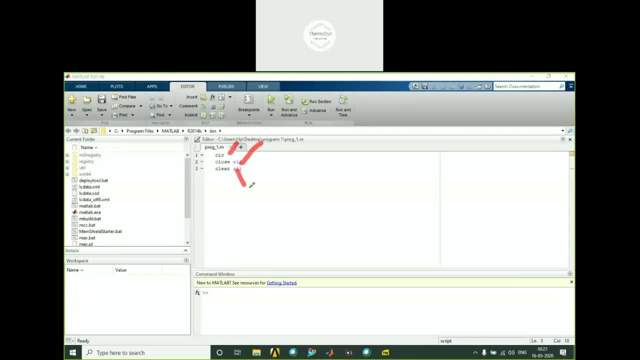 the third one is clear, in order to clear my workspace. okay, guys. so whenever you are running a new program, you should be clear that your matlab background is clear. okay, because in one program you may define a equal to 10, in another program you may define a equal to 15.. what happens? 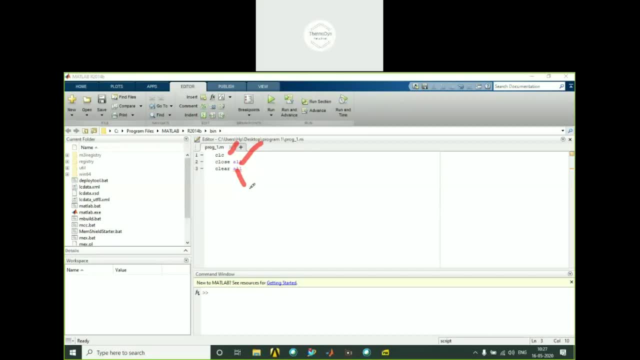 if, uh, you know, in the name of a uh, the thing has two values, so what value does my uh formula will take? okay, so there will be a lot of trivial kind of stuff. okay, so, in order to avoid all uh, you are going to use a clc: close all clear, okay, and um, today we are going to solve a program which will 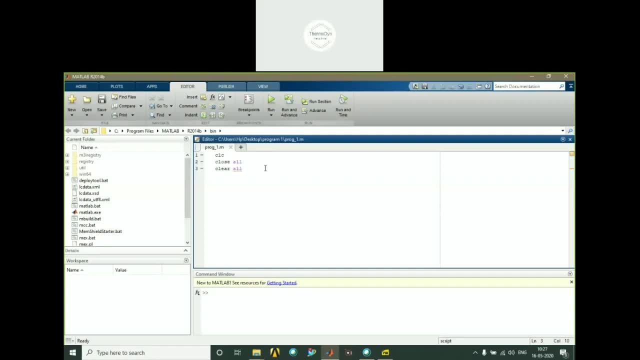 have you know, maximum of 15 or 20 lines only, practically in industry, in a CFD and all, we write codes which will have hundred, two hundred, three hundred, even more than those. okay. so, while writing codes of that much length, you know we face the issue of sorting out the codes, okay so, 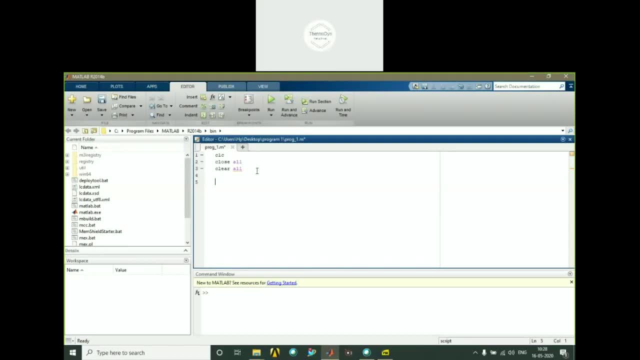 we don't know from where what came. like that, you'll be confused. so, in order to avoid all those, we have to segregate and write up the program. okay, so in order to segregate all the stuff and in order to give command, a command to understand all. 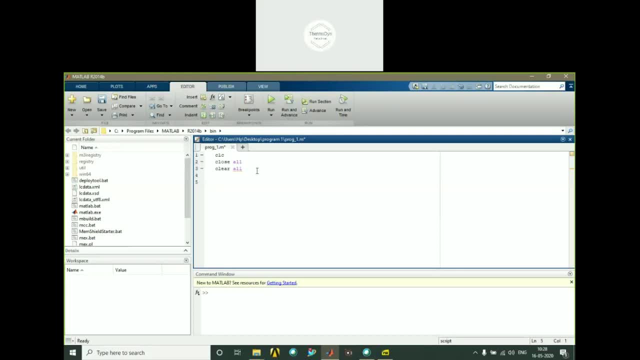 those stuff. we use two things, once double percentage, another one is single percentage, double percentage. we used to section, okay, so you, we used to section the probe problem. it is like input block, computation block, output block, double percentage, double percentage, double percentage, okay, so I'll define like input block, so likewise, whatever value you define. so 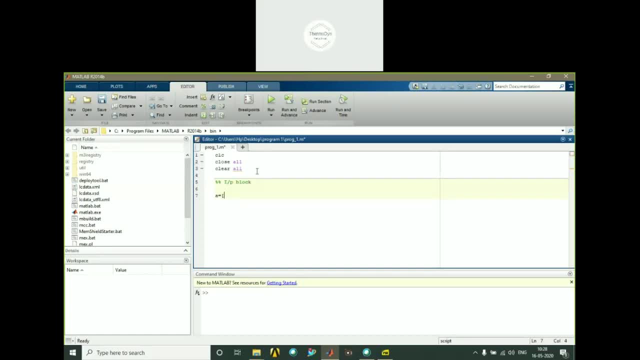 what I do is I'll define a equal to one space two space three and four space five space six. okay, so I'm just trying to define a matrix, okay, guys. so in the input block am just trying to define the matrix. okay, so this matrix is of size 3, cross 3. okay, 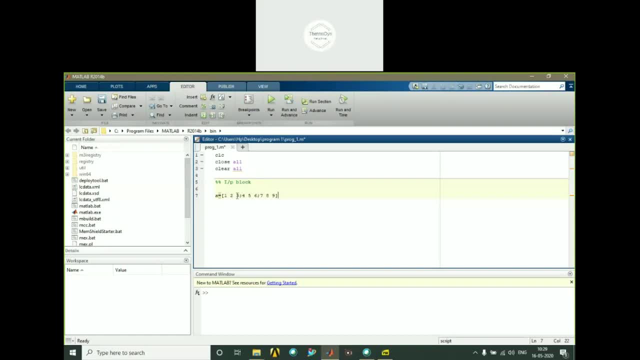 so, guys, in order to define the matrix, you are supposed to use square bracket and in order to segregate the rows and column: in order to separate the column, you are going to use space, or else you can use comma. in order to separate the rows, you are going to use semicolon. okay, so I will show you what happens if. 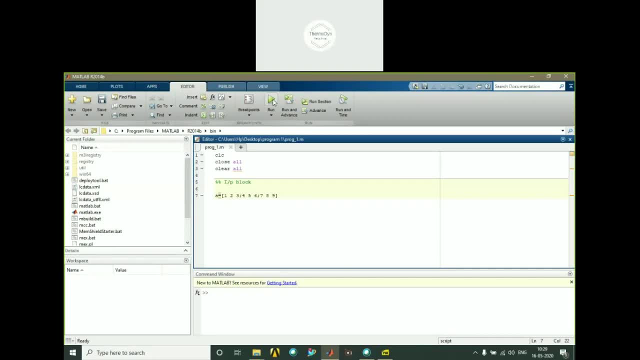 my run this program. okay, so just run it over here. change folder guys. please look at the bottom. we have the: a matrix of 3 cross 3. okay, a matrix of 3 cross 3. so, as you can see, in the left side we have the workspace in which. 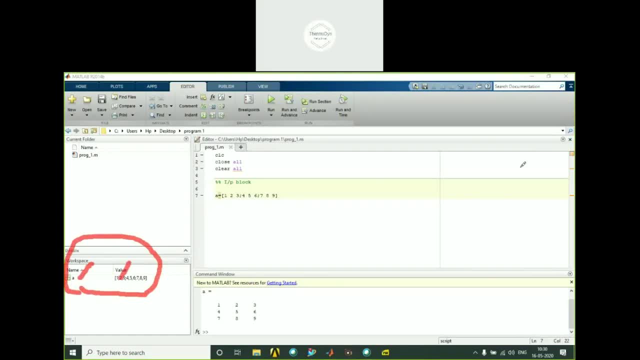 the values have been defined to the a. okay, very, very simple, okay. so in the input block I have defined this stuff. guys, I also want to show you something, because whenever I define something, like I want to define b equal to okay. so I have two steps: a equal to some matrix, b equal to some matrix- okay. so now I am going. 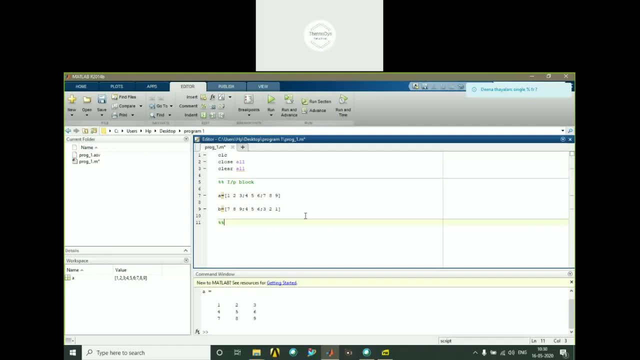 for computation block. it's like a basic arithmetic operation, so I will use double percentage. yes, Dhinadharan, you can ask me. yes, I'll tell you. please be patient. okay, so computation block. so what I'll do is I'll define a variable C, which means a plus B. okay, so if you run this, what? 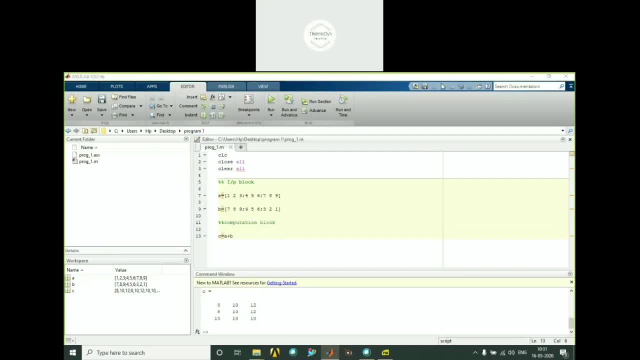 happens is you will have your new variable, which is the addition of first two, a and b. so what I wanted to tell you is, if you're going, the command I will see like: a equal to this, B equal to this, C equal to this, everything will we echo. 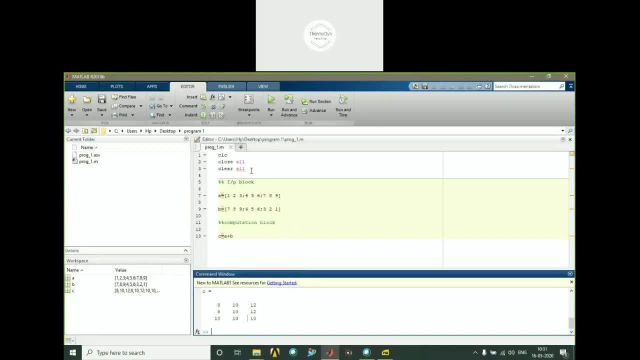 each and every time it will get reflected. okay, and what happens if I remove this? okay, what? what happens if I remove this? guys, please see, if I run it- see here I will get a equal to again I will get. so all the history will be there. if I run for three times, you will get the stuff for three times. okay, that is because 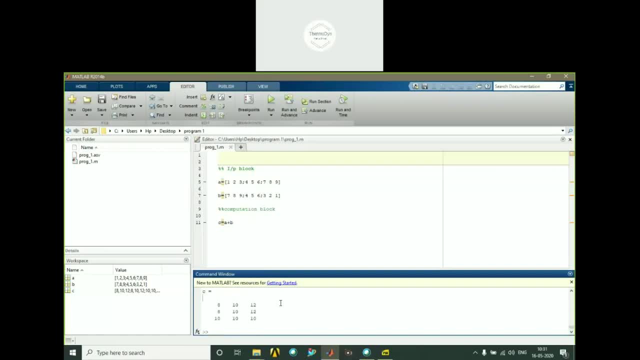 my history have not been cleared. what I, what do I mean by history? clc: clearing the screen. if I use clc here, if you run it, you will only see one: a, b, c, nothing else. okay. so this is the importance of clc: it will clear your command window from your old junk. next one is how to 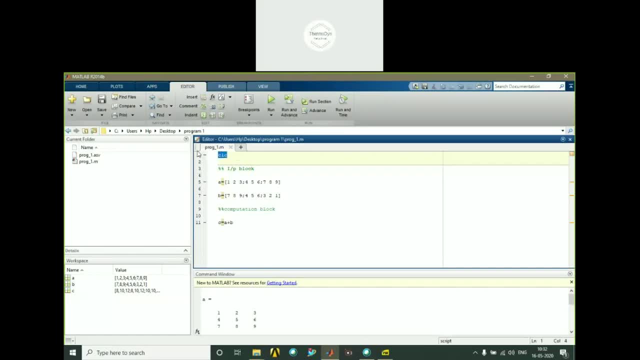 you know, clear your workspace. in order to explain that, I will use my command window. guys, please see, we are seeing in depth. okay, so all these stuffs are very important as a beginners you. so, in order to clear my workspace as you can see here, I will have- I'm having three- 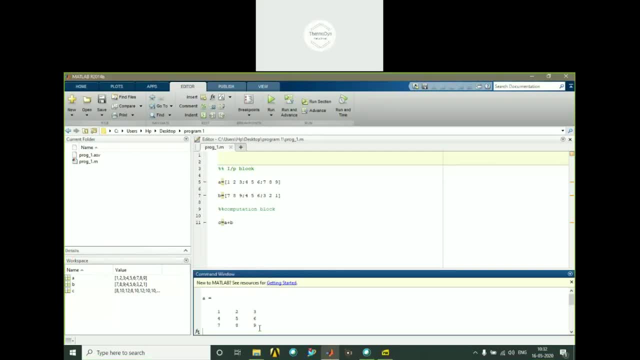 matrixes. okay, I'm having three matrices in order to clear all, just type clear. all what happens is: now my workspace is cleared. okay, my workspace is clear, nothing is there. so, likewise, I can close all my unnecessary windows by using close all command. okay, currently I don't have anything to. 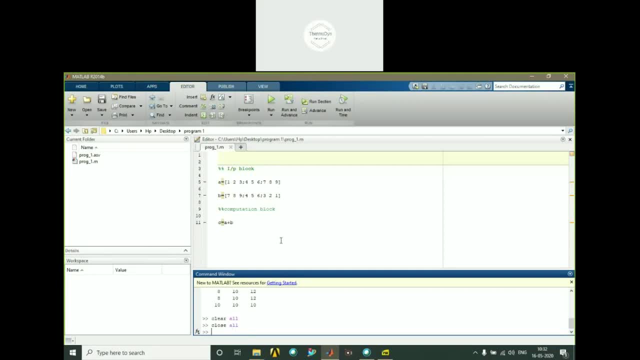 close. but still, if you close all, all the unnecessary windows, you will see that I have stuff. if anything was there, it will get closed. okay, so each time I cannot run these things, you know, individually. that is why I have included all these stuffs in the beginning of my program. okay, so close all and clear all. okay, so you can. 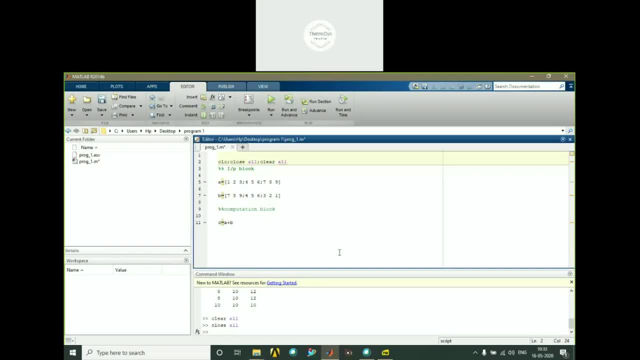 define it one by one, or else you can use semicolon to define multiple roles at the same line. okay, guys and guys, please listen. I hope you are taking a note, please listen. you know so if I run this I have ABC, but most of the time we don't. 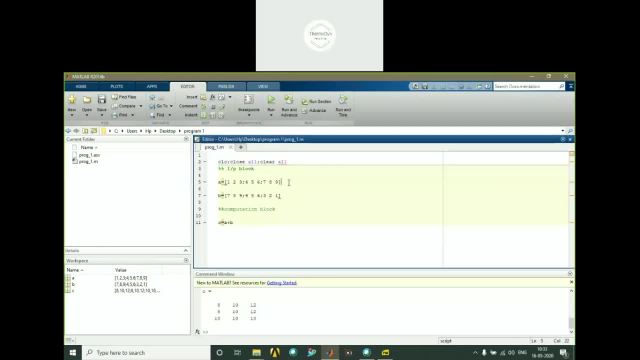 want the input because we know the input. we only need the output. in order to suppress the input, please use semicolon behind each and every line. okay, if you use the semicolon and if you run it, please see here, even if I scroll, I will only have my output. okay, so I will not get. 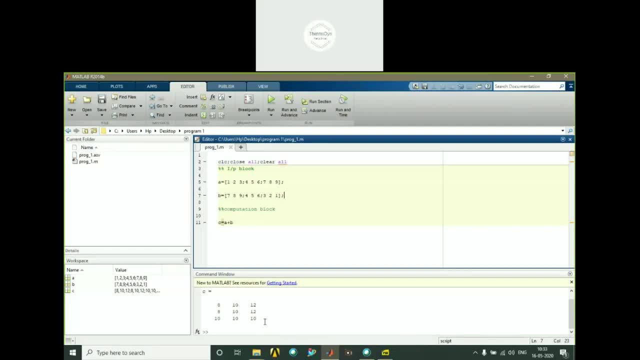 echo of what is A, what is B. only I will have a value of C matrix. okay, guys, so I have defined my input block, I'm defined, I have defined my computation block. since this is, you know, matrix operation, there is no need for us to go for output. 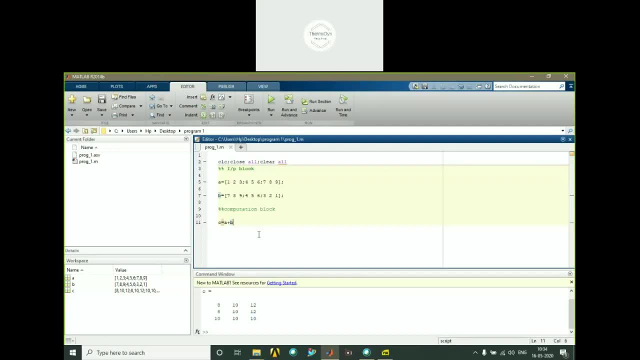 block and all, because we don't have. there is no need for us to create graph and all. I will show you those things in the next thing, as you ask Dean Adhayan, what does single percentage means? single percentage means command. okay, because this particular code has only two inputs, but I'll show. 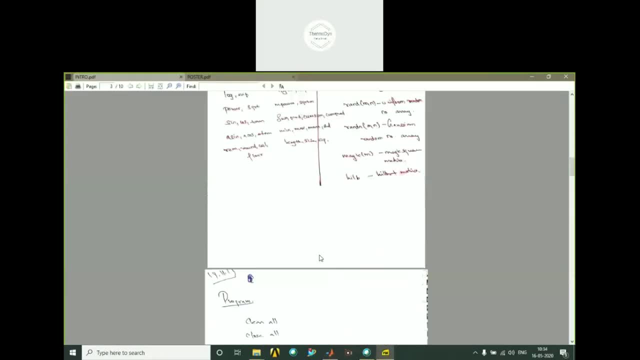 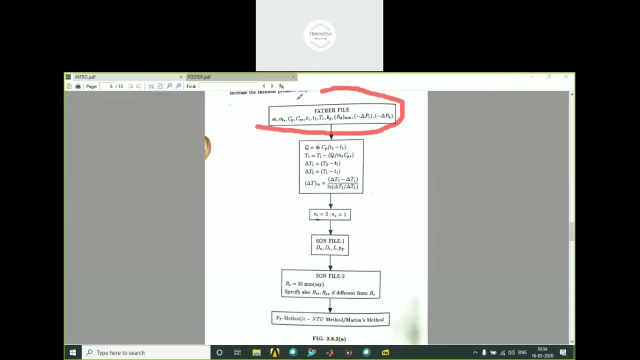 you something. so you know this is the typical, very old syntax which is used of FORTRAN programming. okay, so when you see here as a father file, Input file will have so many inputs, so many inputs, so many formulas, so many if-else loop while loop, so many sun files, which means output file. 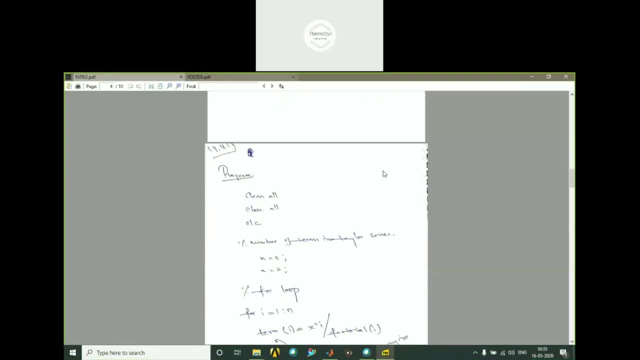 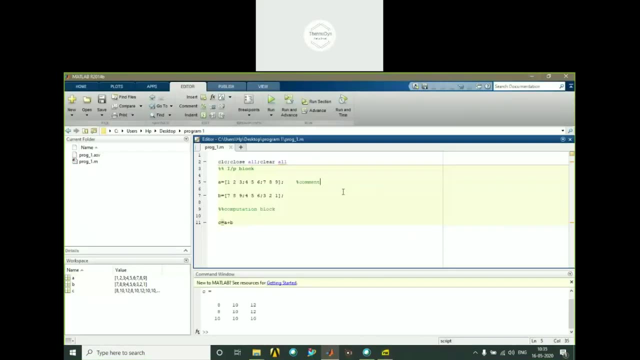 So when you have so much kind of stuff, what happens is you don't know what means what, And while writing a code which is of signal processing or heat transfer kind of stuff, we have to define the units. That is very, very important because the whole company will somewhat depend on your program. 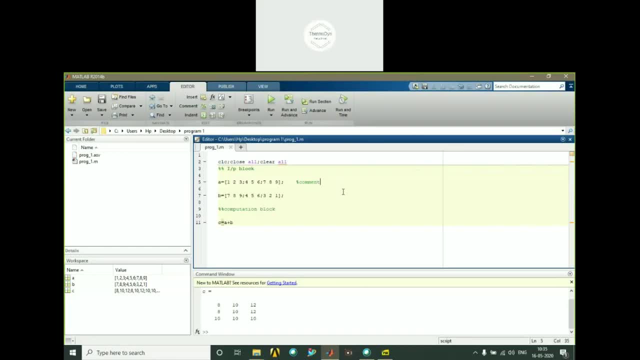 Everybody uses different units, So you want to point out in which unit you have wrote your code. So, in order to define that, after each input you are supposed to give your units. So when you use single percentage or double percentage, MATLAB is not. 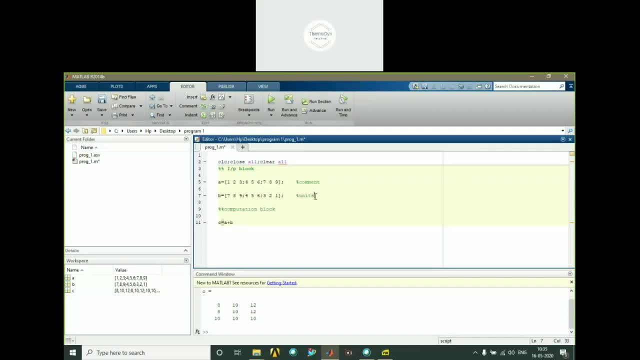 It is not going to run that particular line. So if you use single percentage, that is command. if you use double percentage, that is sectioning. And what I am going to now is I am going to increase my size, matrix size, to show you the power of MATLAB. 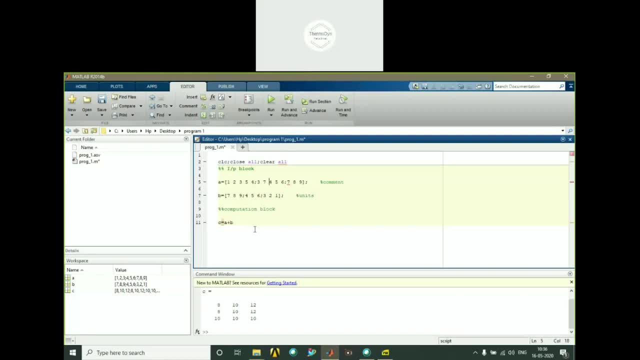 So I am going to give my matrix size 1,, 2,, 3,, 4,, 5, S. Okay, so now I have a matrix of 5 cross 5 in A. You know, guys, I am just using random number. you can also try. 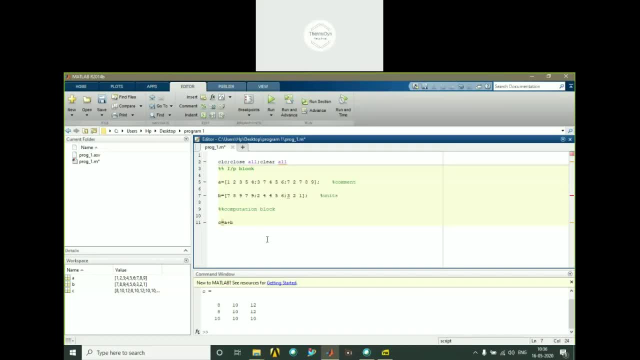 Okay, Okay, Now I have a matrix of 5 cross 5.. If you run, you will see that. sorry, small issue, I have to add some more lines. Sorry, small issue, I have to add some more lines. 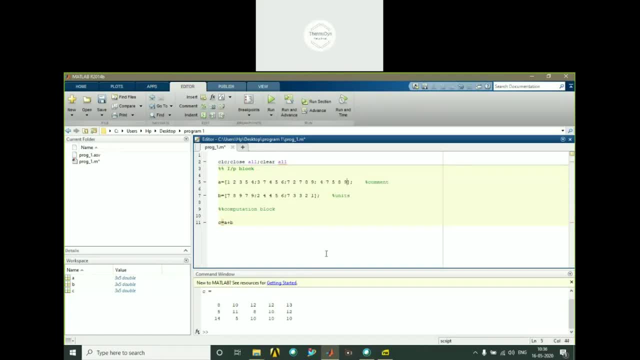 Okay, S Yeah, Next likewise over here. Next likewise over here. 1, 2,, 3,, 4, 5, S. 1, 2,, 3,, 4,, 5, S. 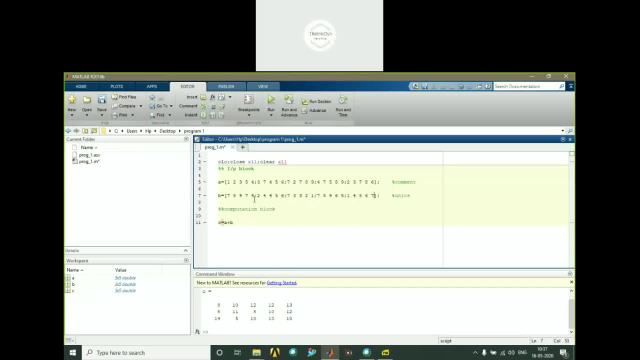 Yes, So if you run it, you will have a matrix of 5 cross 5.. You will have a matrix of 5 cross 5.. Good, Okay, Yes, guys. So, as you can see, whatever your matrix size is, 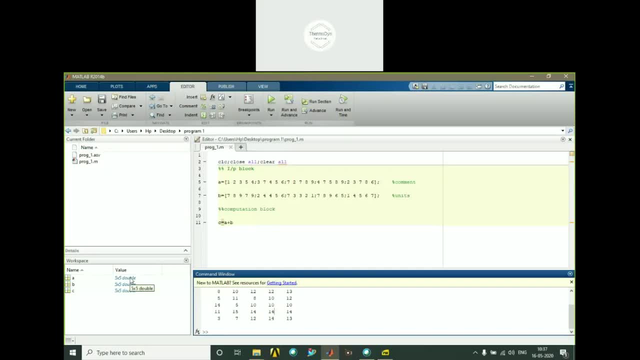 Okay, Why? Because if you want to see your matrix in, you know like Excel kind of stuff, just double click over here. Because if you want to see your matrix in, you know like Excel kind of stuff, just double click over here. 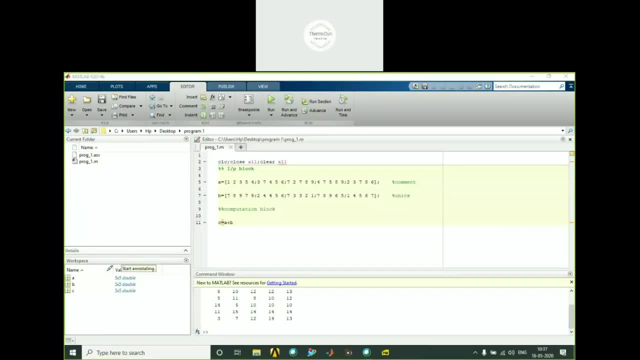 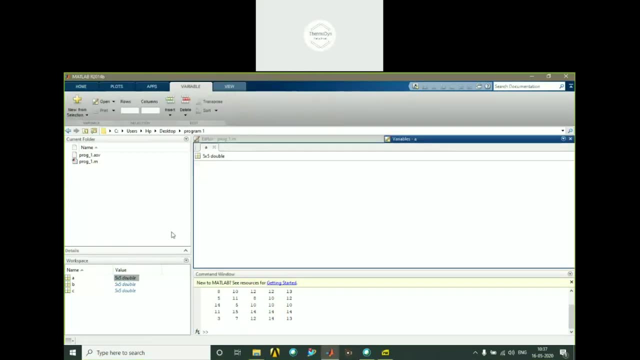 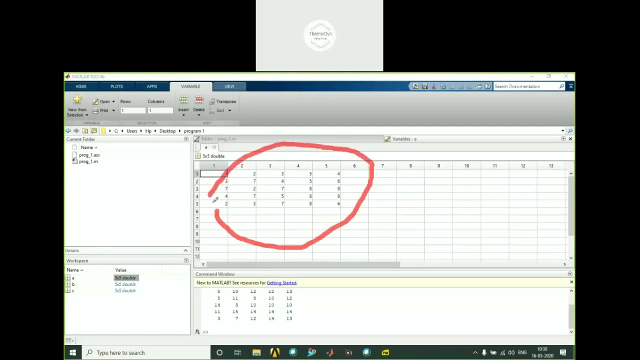 here, guys, please see, to the left of your screen, you will have all those values: 5 cross 5, 5 cross 5, everything. okay, so if you just double click it, a window will open. okay, so, as you can see, this particular excel sheet will carry all. 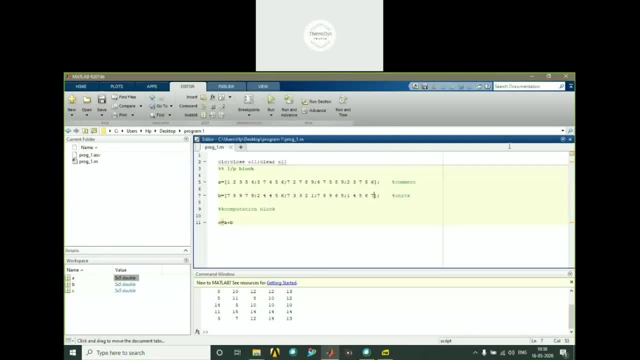 your data. okay. so what happens if I want to carry out a multiplication operation, because addition is somewhat simple, but in order to multiply this two- you know A and B matrices- generally manually, it will take 45 to 50 minutes. okay, I am very sure. okay, because if you are, if you are aware of matrix multiplication, then 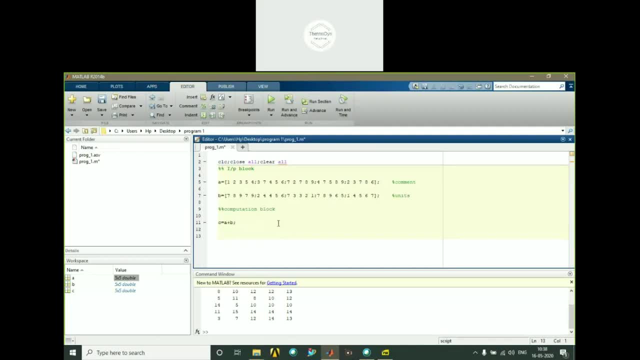 you can just assume the complicity, even after taking 40 minutes. definitely, I am telling you you will have at least of 5 errors, 5 number errors, okay. so if you want to have a multiplication of this, two D, equal to A multiplication of B, okay. 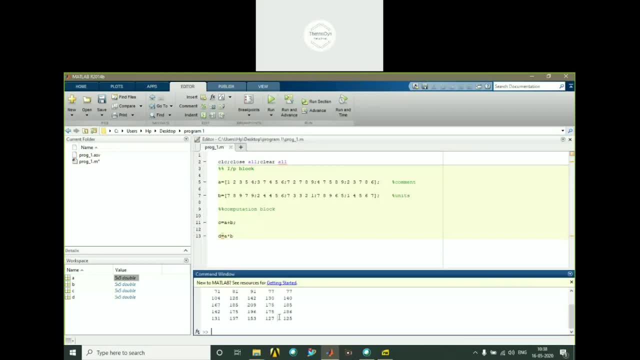 okay, so just run it, you will have multiplication of those in. I hope you know some one second like that. okay, so very simple guys. so even if you have a hundred cross hundred matrix, you may ask me where I am going to have a matrix of hundred plus hundred. okay, nowadays, a thing called computational methods, it's. 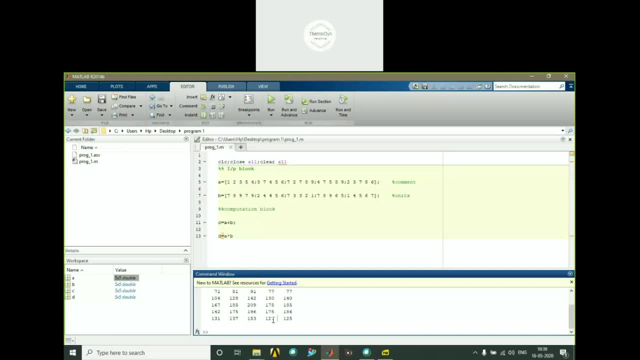 like numerical method. its common for easy, typically mechanical. you know it is a life for mechanical and easy peoples. electromagnetic simulation, error, R o, space marine. you know computational methods are alive. without that you cannot do anything in solving those computational problems. i am telling you, you are going to, sometimes you are going to solve. 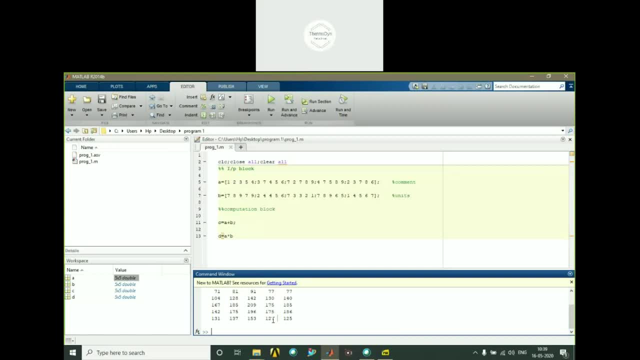 matrix of even thousand cross thousand. okay, that is because of taylor series of expansion where you will have numerous matrices data. okay, so when you assume that time, that much of that much amount of data, it's practically impossible to solve using, you know, manually and if you use python, kind of